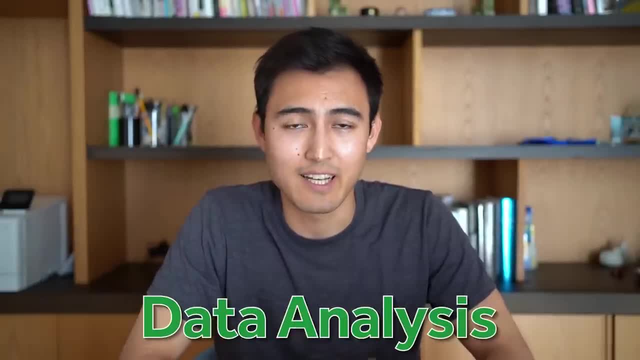 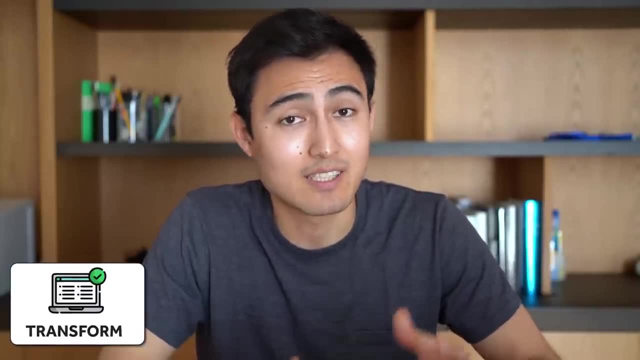 In this video, you're going to learn all the fundamentals of data analysis, and we'll break this down into four main areas. First, we're going to be looking at transforming the data, so cleaning it up. Secondly, we're going to be looking at creating descriptive statistics to 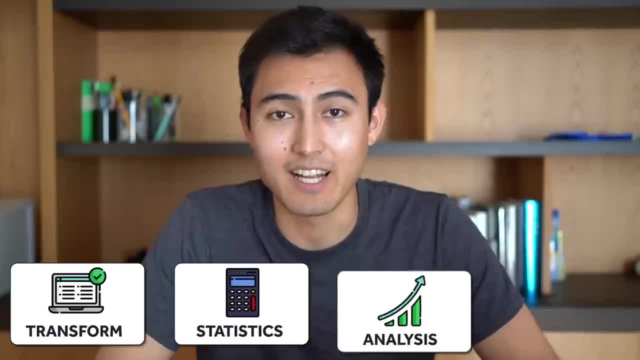 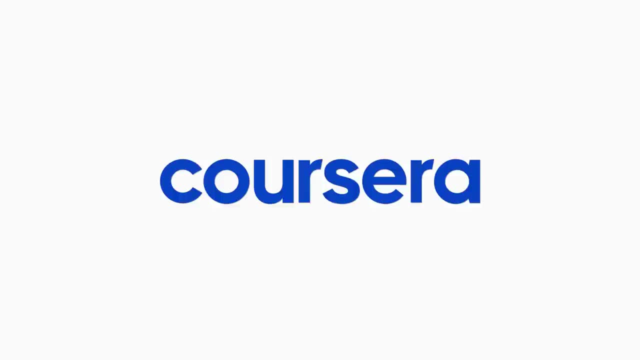 understand it better. Third, we're going to be looking at data analysis And finally, we'll get into creating a report to visualize our findings. So let's get into it, And thank you to Coursera for sponsoring this video. More on them later. The first step here is to transform the 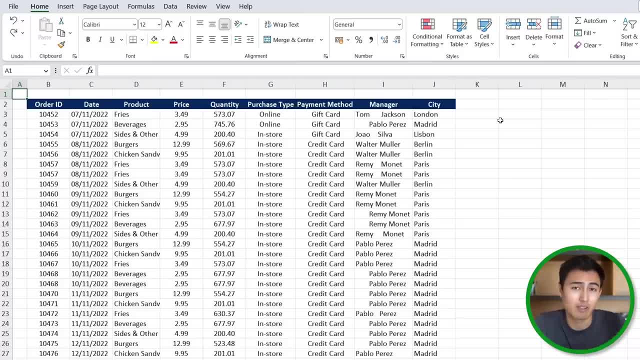 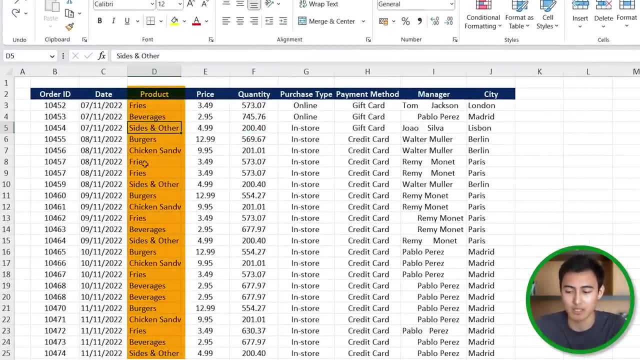 data, And for this, here's the Excel file that we'll be working with, which you can download for free in the video description. So, as you can see, this is going to be for a fast food chain. You can see the types of products here, And the first step is simply to clean this up. 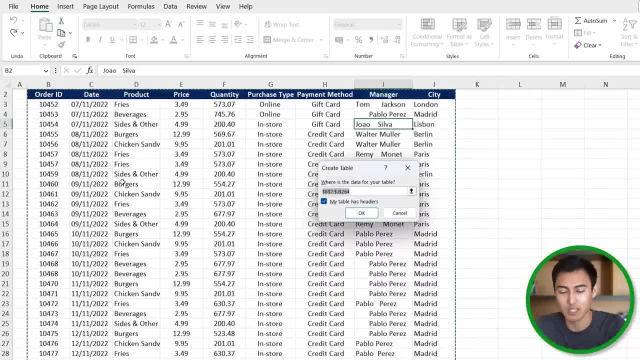 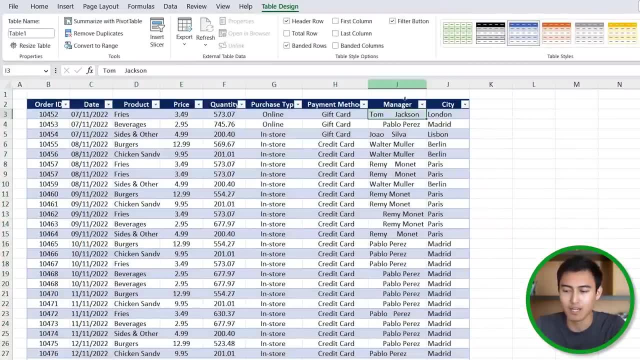 But for that we're going to go to control T, So to change this into a table. so change the data set into a table, Then we'll hit on OK From here for the cleaning that part. you can see that under the manager column we seem to have some very odd spacing. 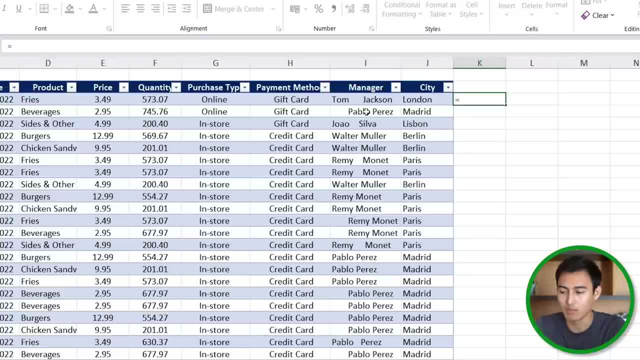 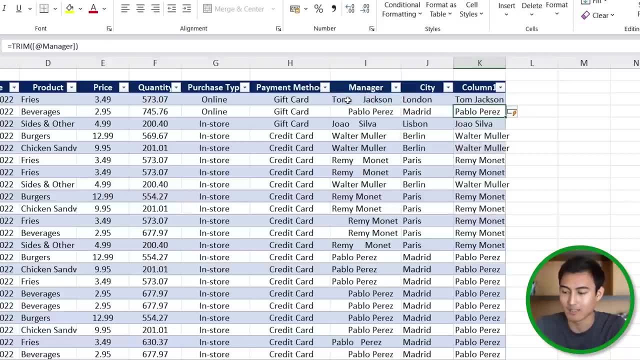 here. So let's go ahead and clean that up here. We're going to go to equals trim, hit the tab key And this formula is going to remove these odd spaces. We'll hit enter. there You can see that's going to auto populate for all of these. We'll change this name to manager. 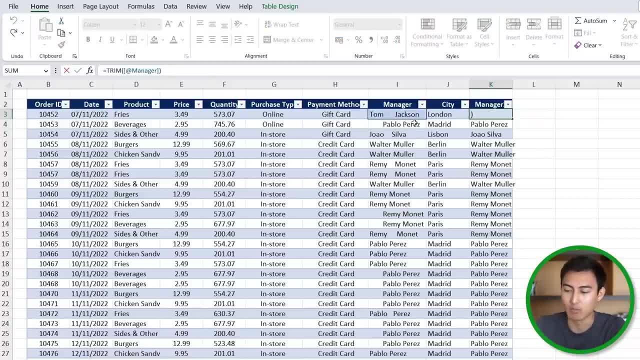 And then, for all of these that are currently linked to this column over here, we're going to paste them as values, So we're going to go control change. and then we're going to paste them as values, So we're going to go control. 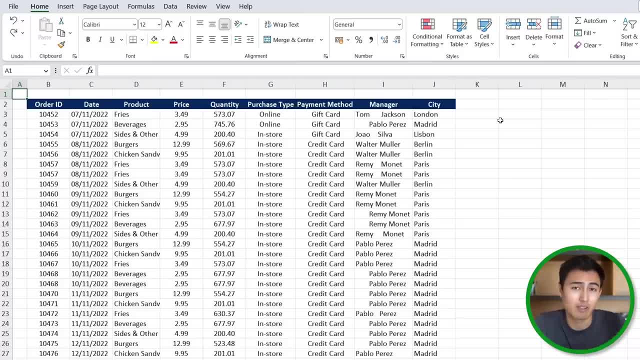 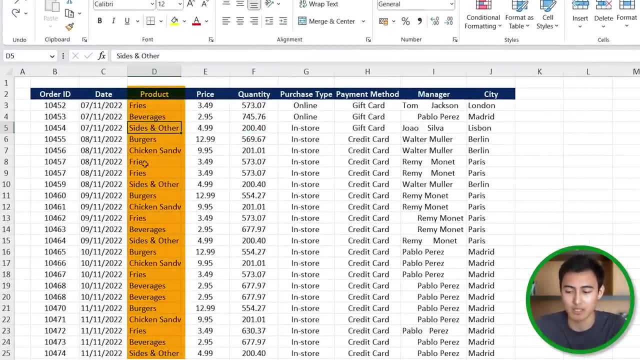 data, And for this, here's the Excel file that we'll be working with, which you can download for free in the video description. So, as you can see, this is going to be for a fast food chain. You can see the types of products here, And the first step is simply to clean this up. 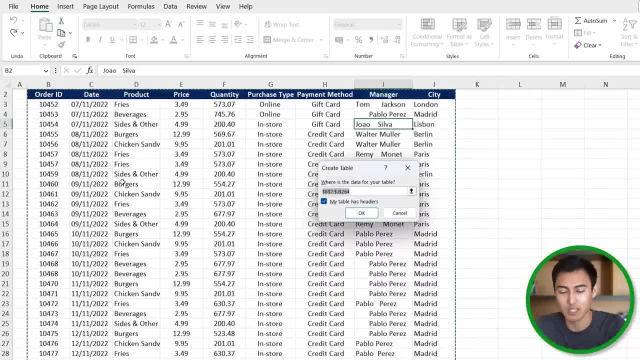 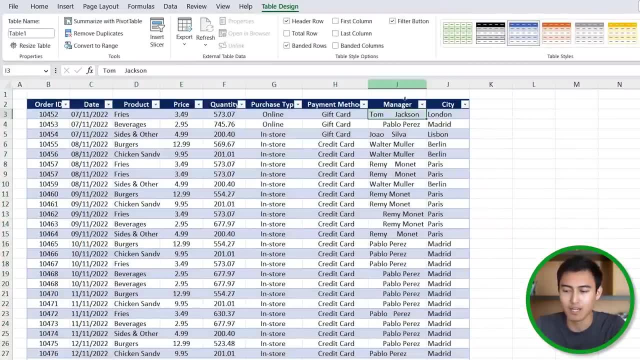 But for that we're going to go to control T, So to change this into a table. so change the data set into a table, Then we'll hit on OK From here for the cleaning that part. you can see that under the manager column we seem to have some very odd spacing. 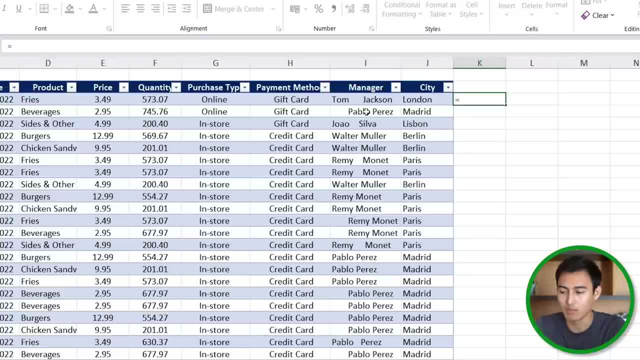 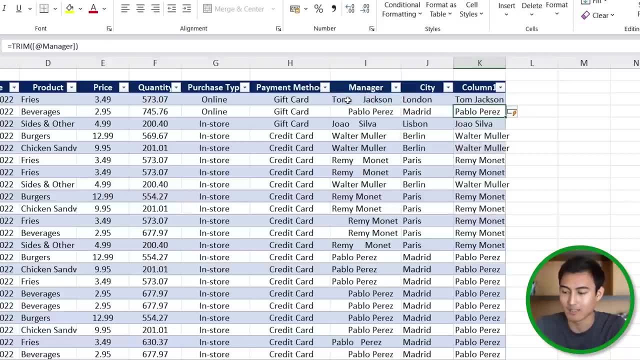 here. So let's go ahead and clean that up here. We're going to go to equals trim, hit the tab key And this formula is going to remove these odd spaces. We'll hit enter. there You can see that's going to auto populate for all of these. We'll change this name to manager. 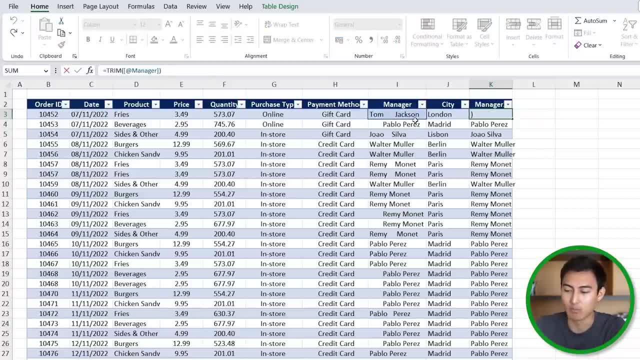 And then, for all of these that are currently linked to this column over here, we're going to paste them as values, So we're going to go control change. and then we're going to paste them as values, So we're going to go control. 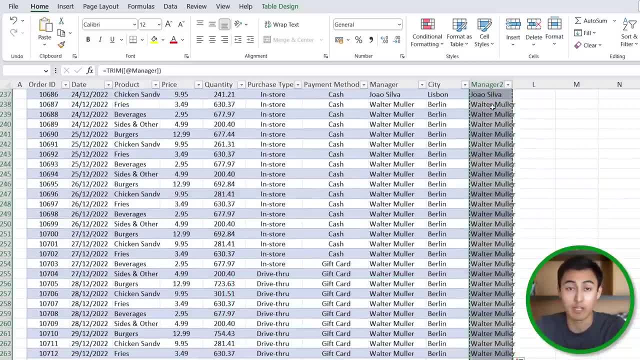 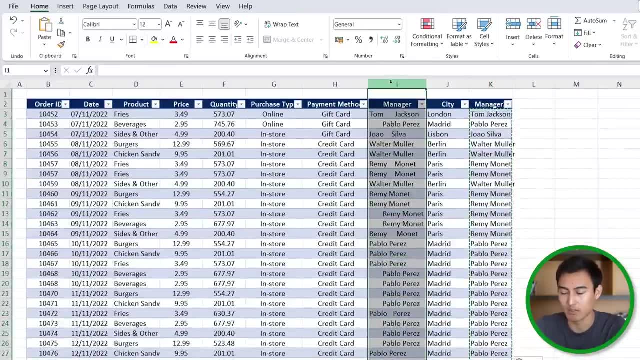 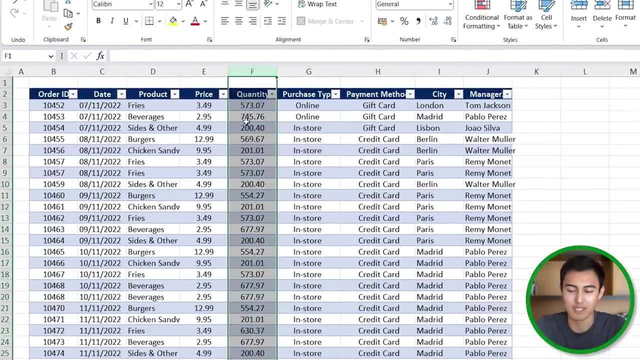 shift down control C And then we're going to paste these as a value. So alt H, V, V is a shortcut for that, And now that means that we can go ahead and remove this column by hitting control minus. There you go. Then under quantity you might notice that we've got these decimals. 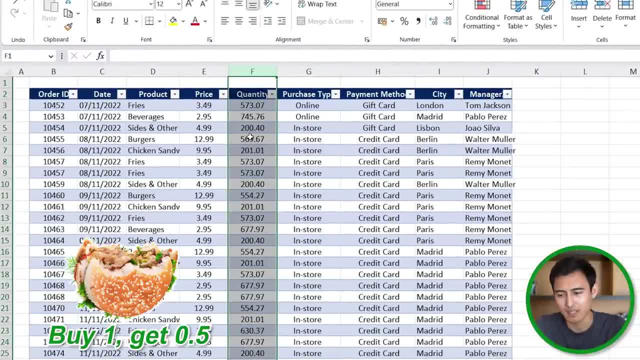 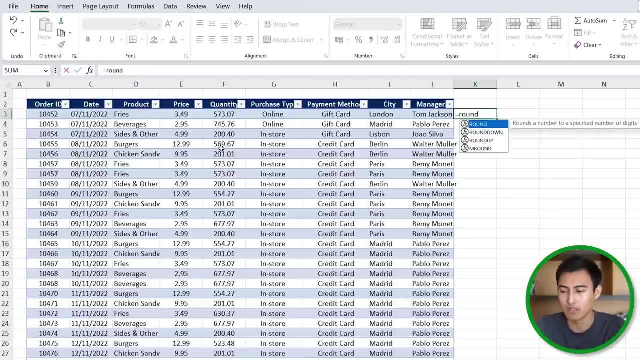 which don't make too much sense. You can't really have half a burger, And so for this we're basically going to have to round up to a whole number. For that we're going to use the roundup formula. So equals round up. 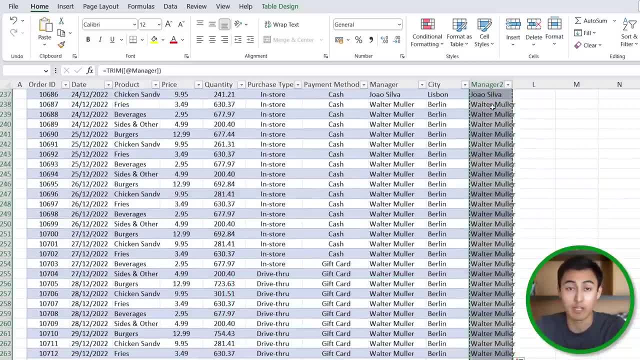 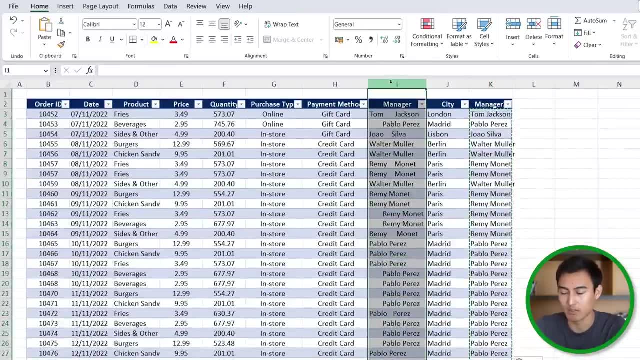 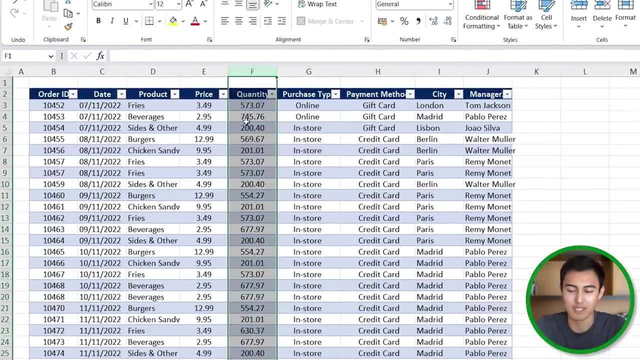 shift down control C And then we're going to paste these as a value. So alt H, V, V is a shortcut for that, And now that means that we can go ahead and remove this column by hitting control minus. There you go. Then under quantity you might notice that we've got these decimals. 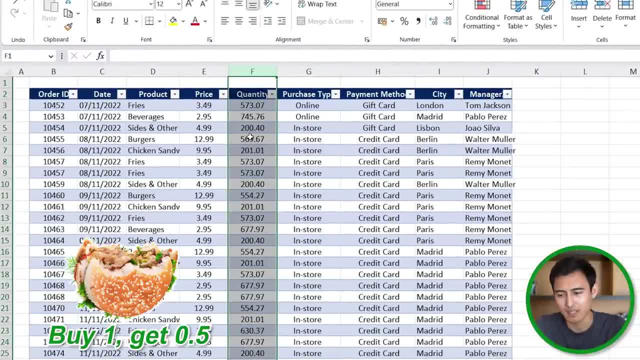 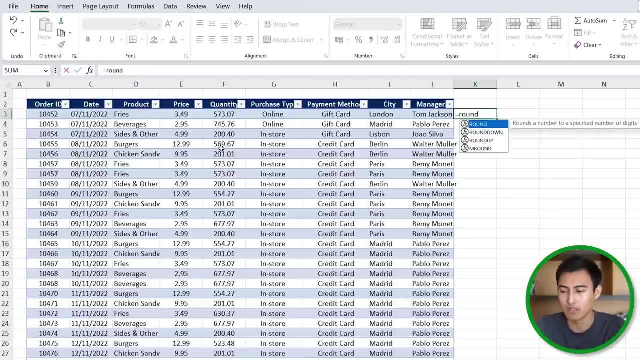 which don't make too much sense. You can't really have half a burger, And so for this we're basically going to have to round up to a whole number. For that we're going to use the roundup formula. So equals round up. 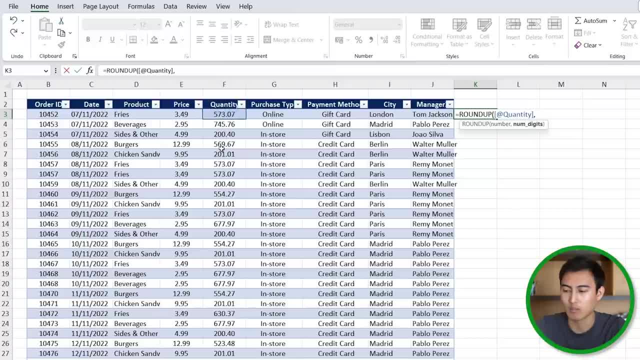 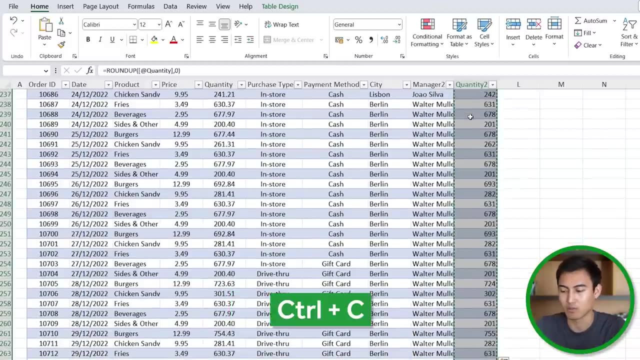 Hit the top key there, The number is this: one comma, And the number of digits for us is going to be zero because we want the full number. Close those brackets and hit enter. So this is going to be our quantity now Hit enter there And we basically want to control, shift down, control C. 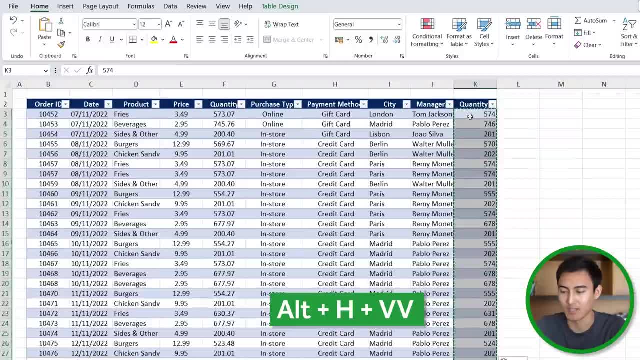 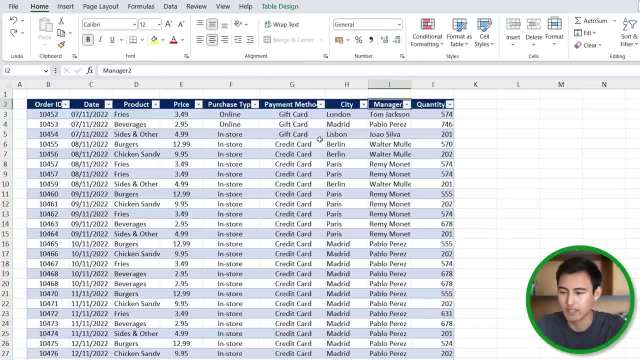 and then paste as values. So alt, H, V, V again. There you go. So now we can remove this column here. So we're going to select it and control minus. Then you'll notice that under city here we have the city names, but we don't necessarily have the countries. 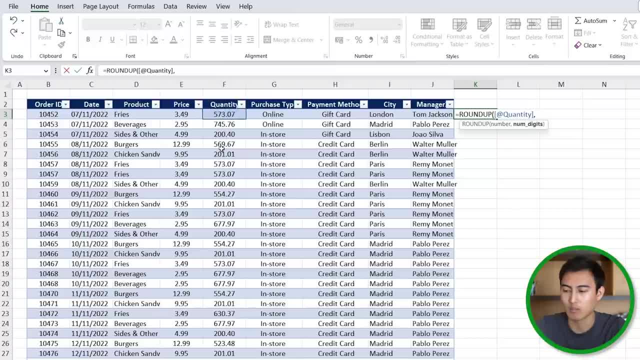 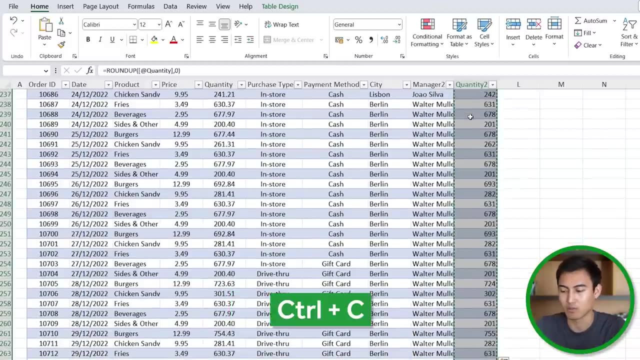 Hit the top key there, The number is this: one comma, And the number of digits for us is going to be zero because we want the full number. Close those brackets and hit enter. So this is going to be our quantity now Hit enter there And we basically want to control, shift down, control C. 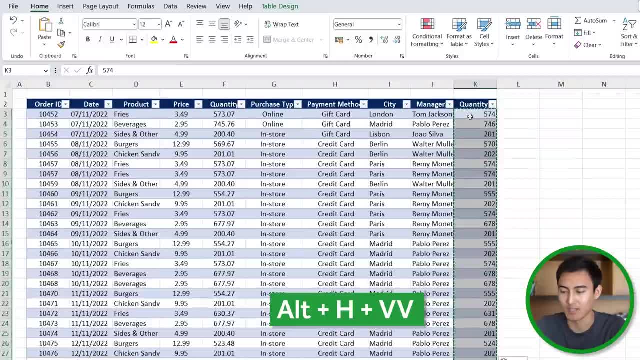 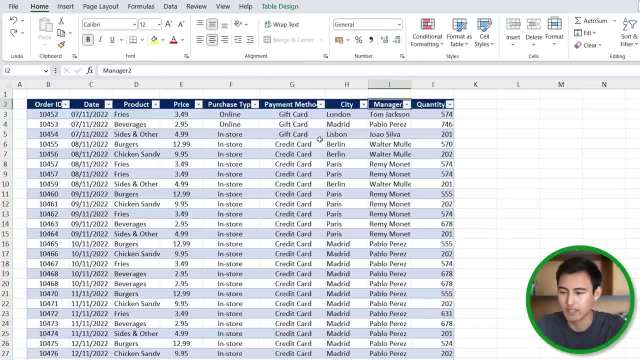 and then paste as values. So alt, H, V, V again. There you go. So now we can remove this column here. So we're going to select it and control minus. Then you'll notice that under city here we have the city names, but we don't necessarily have the countries. 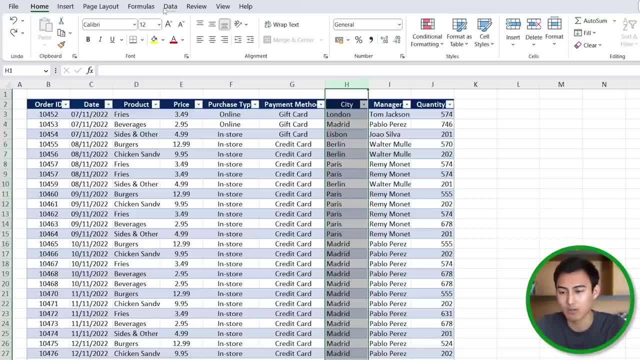 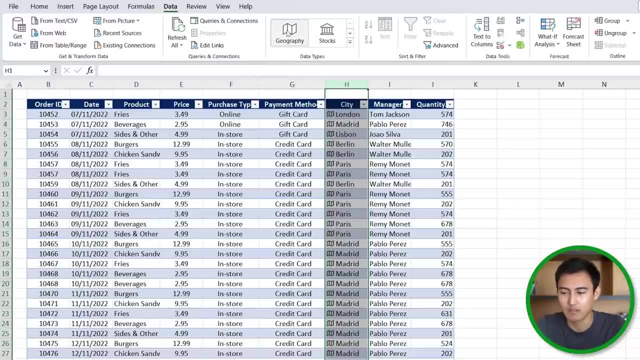 That would be a nice thing to add. So for this, we can actually head over to the data tab and go under data types. You'll find geography here, So just click on that. Once you start to see that icon, it means that it's loaded up. What you want to do here is hit. 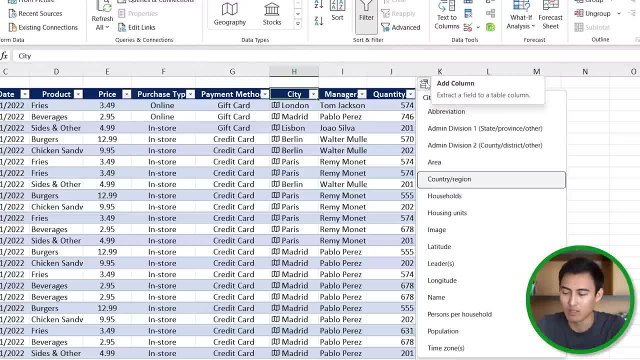 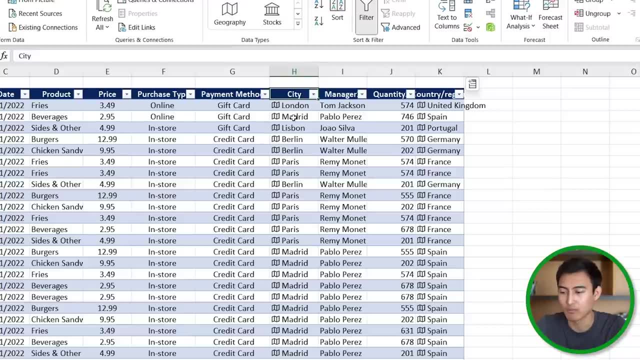 over to this icon to the side under add column, And we basically want to add a country or a region associated with that city And you can see that we have the country name here. So we're going to just move the corresponding country for each city. If you want to move this city column next to the 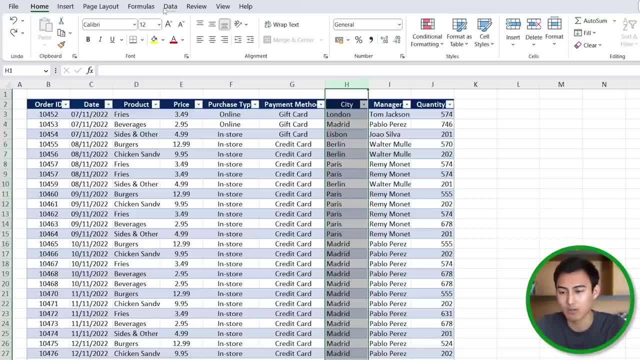 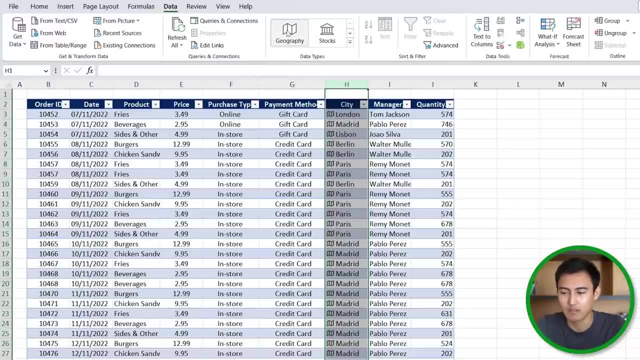 That would be a nice thing to add. So for this, we can actually head over to the data tab and go under data types. You'll find geography here, So just click on that. Once you start to see that icon, it means that it's loaded up. What you want to do here is hit. 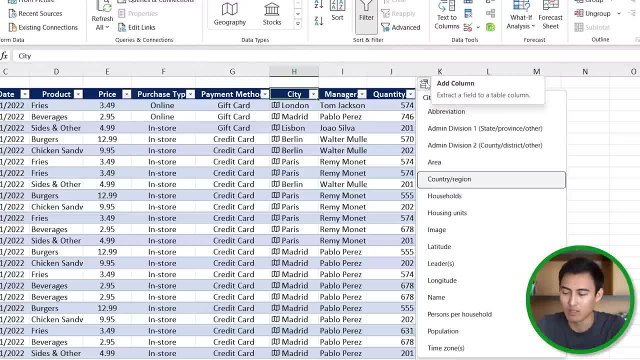 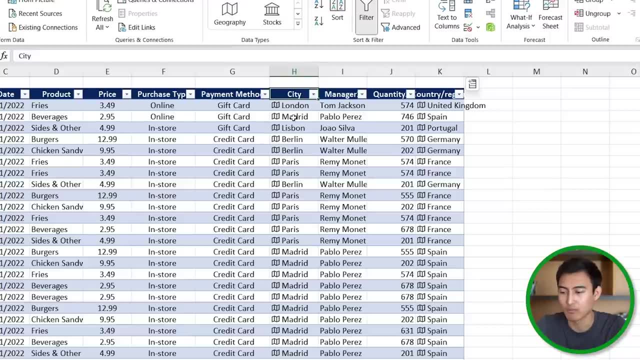 over to this icon to the side under add column, And we basically want to add a country or a region associated with that city And you can see that we have the country name here. So we're going to choose the corresponding country for each city. If you want to move this city column next to the 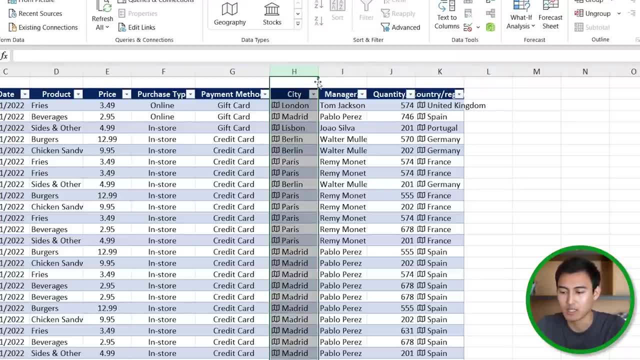 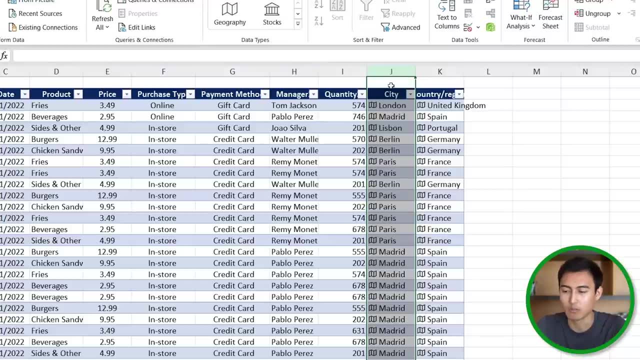 country. you can actually go ahead and select it up top And when you start to see these arrows, when you hover over it, just press a shift key and then just drag it across, like so that should allow you to move everything. One final thing we haven't done here is test if there's any duplicates. 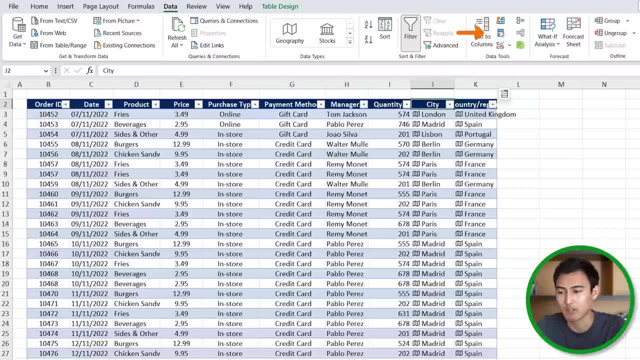 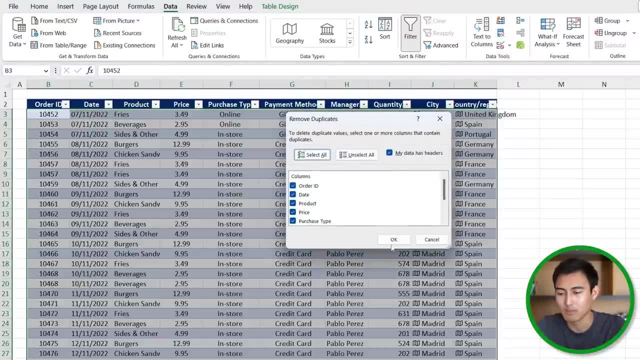 So for this we can simply go under data again and we're just going to remove duplicates by going to this icon over here. So we'll click on that and it's going to be for that whole, that whole table, and we'll simply hit on ok and you can see here that we get a notification saying: 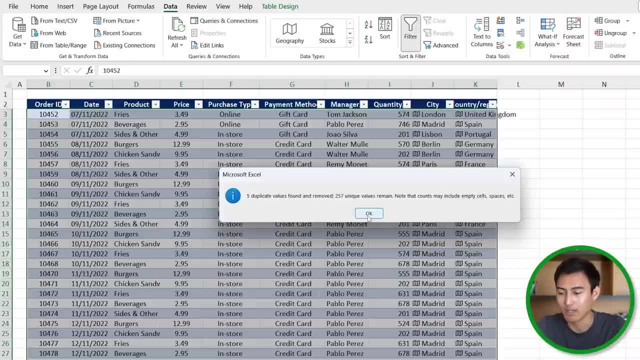 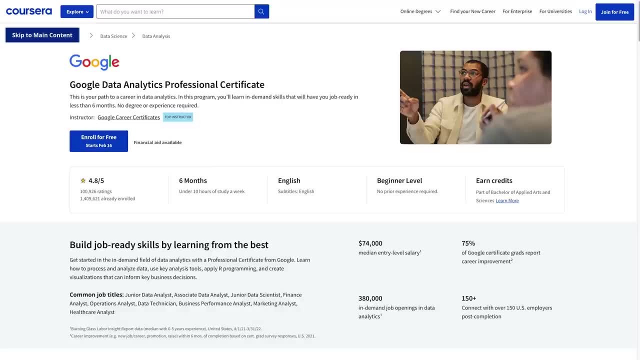 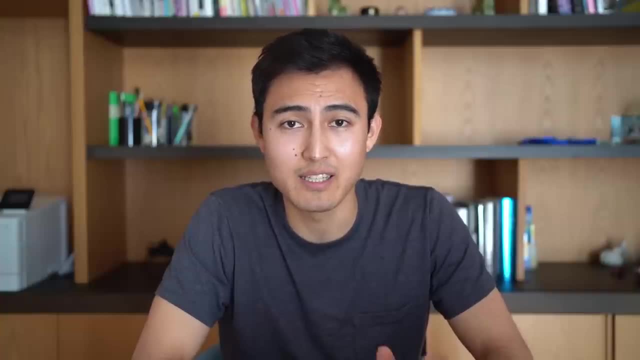 that five duplicate values were found and removed, so we'll hit on ok there. and speaking of data analysis, if this is something that you want to learn more about, you can check out google's data analytics professional certificate. it's designed to teach you job ready skills for any data analytics. 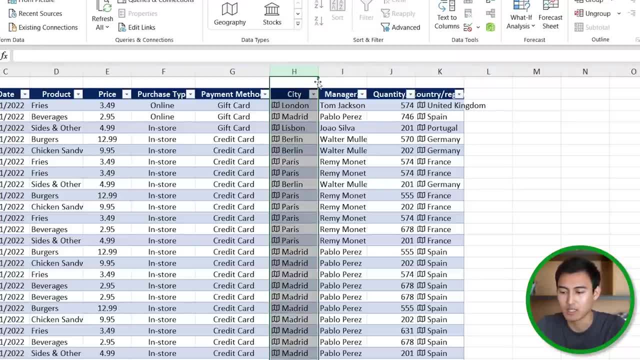 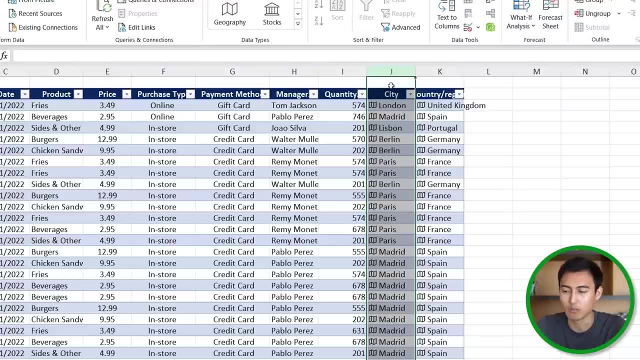 country. you can actually go ahead and select it up top And we start to see these arrows When you hover over it. just press the shift key and then just drag it across, like so. that should allow you to move everything. One final thing we haven't done here is test if there's any duplicates. 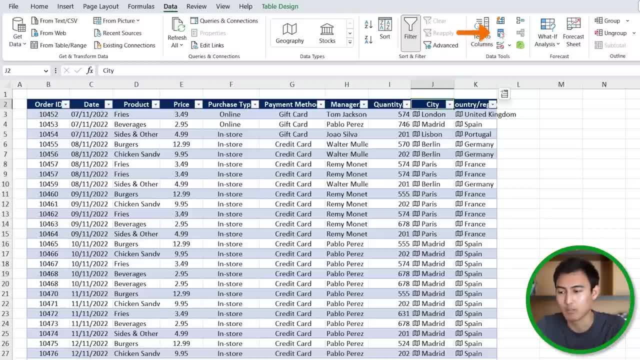 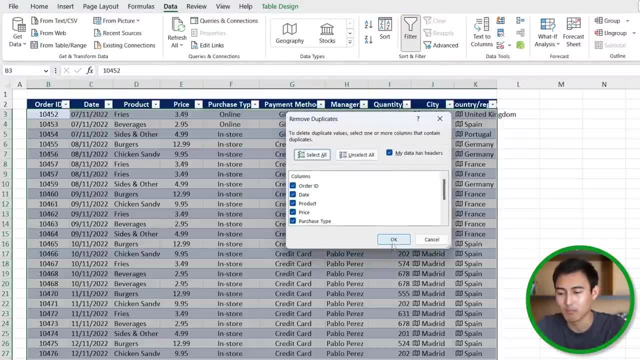 So for this we can simply go under data again And we're just going to remove duplicates by going to this icon over here. So we'll click on that and it's going to be for table and we'll simply hit on ok and you can see here that we get a notification saying that five. 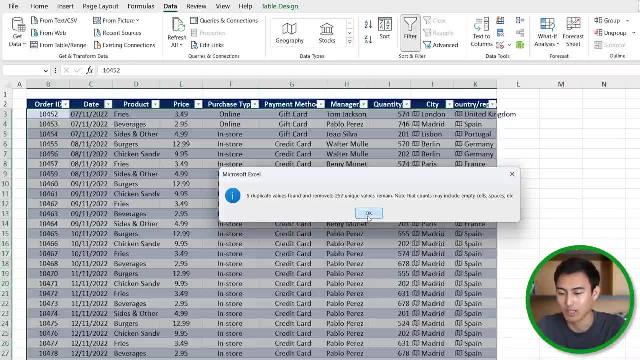 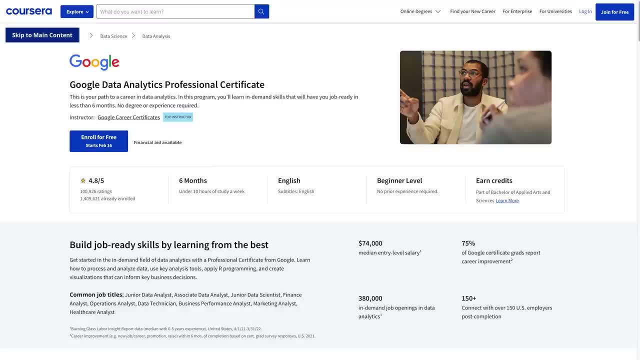 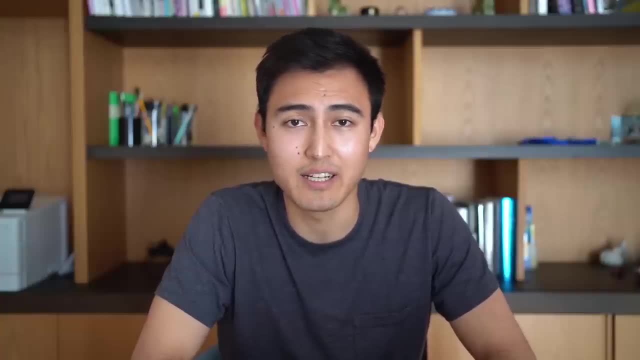 duplicate values were found and removed, so we'll hit on ok there. and speaking of data analysis, if this is something that you want to learn more about, you can check out google's data analytics professional certificate. it's designed to teach you job ready skills for any data analytics role. 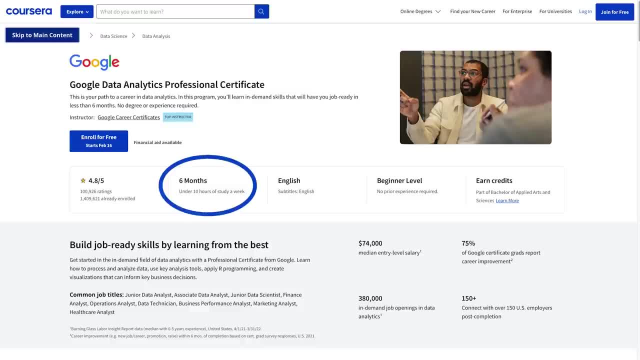 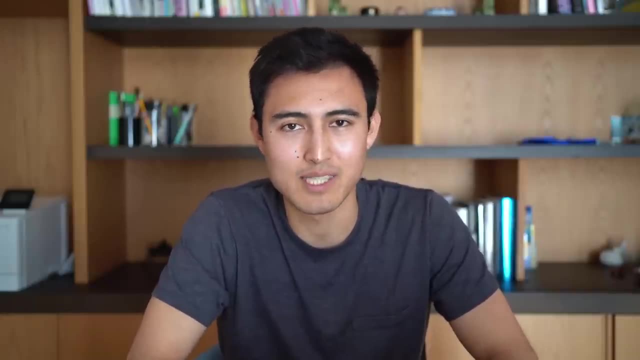 so you can learn all the skills required in less than six months. the program currently has well over 1 million students in a 4.8 star rating. now if you're wondering if you need any prior experience, no, there's no prior experience required and it's all fully self-paced in the program. you learn key 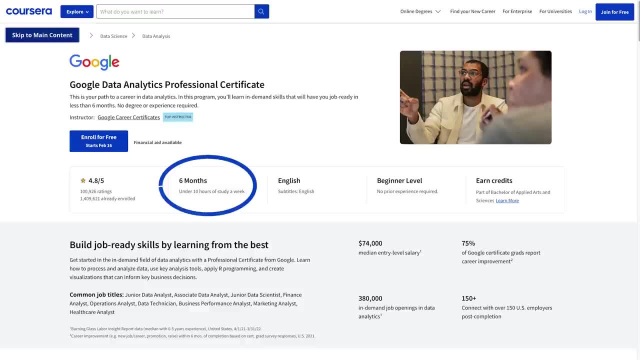 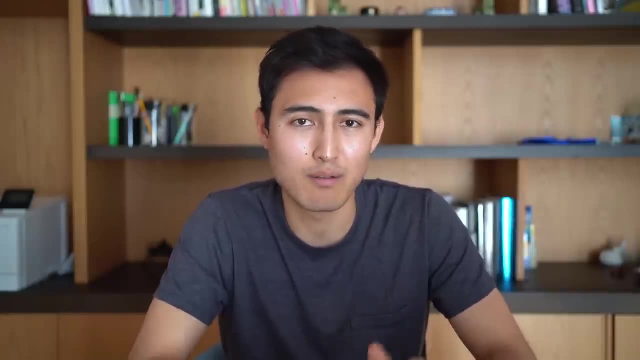 role, so you can learn all the skills required in less than six months. the program currently has well over 1 million students and a 4.8 star rating. now if you're wondering if you need any prior experience, no, there's no prior experience required and it's all fully self-paced in the program. you 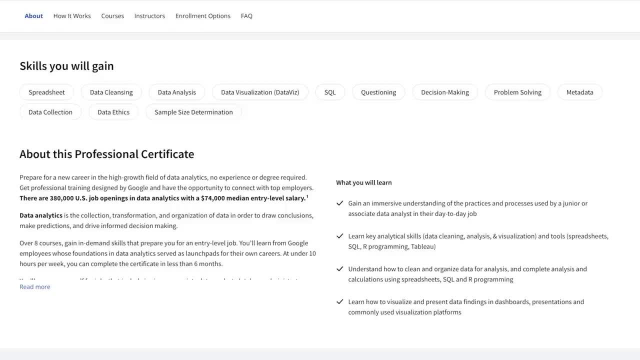 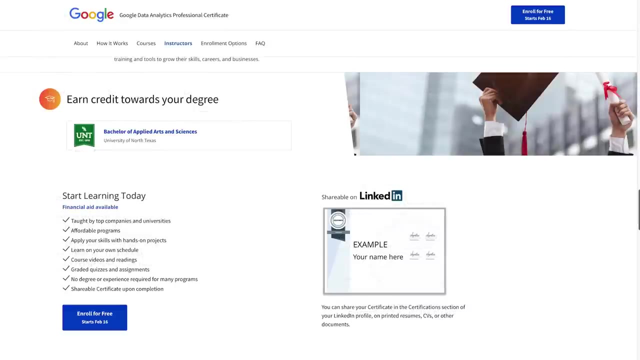 learn key analytical skills, including data cleaning, analysis and visualization, using some of the most common industry tools, such as space spreadsheets, sql or r programming. upon completion, you'll receive a google professional certification which you'll be able to share on your cv and linkedin. so if you're interested, sign up for a. 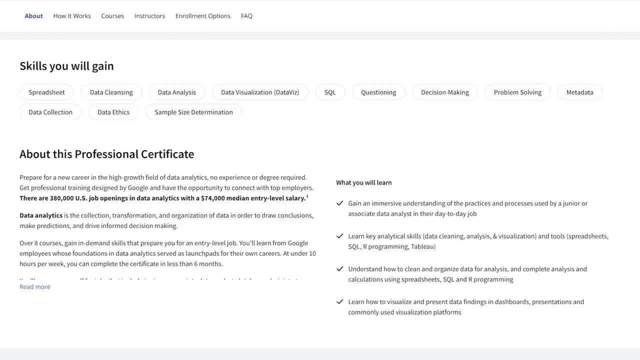 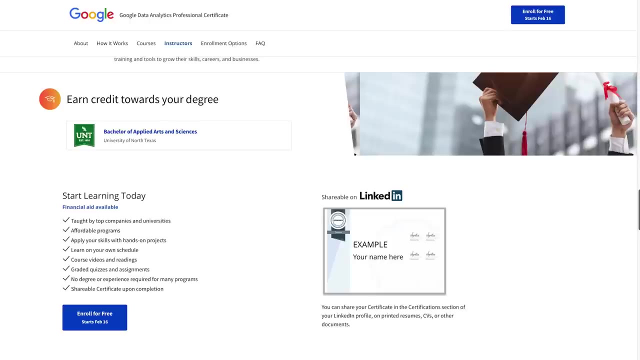 analytical skills, including data cleaning, analysis and visualization, using some of the most common industry tools, such as spreadsheets, sql or r programming. upon completion, you'll receive a google professional certification which you'll be able to share on your cv and linkedin. so if you're interested, sign up for a. 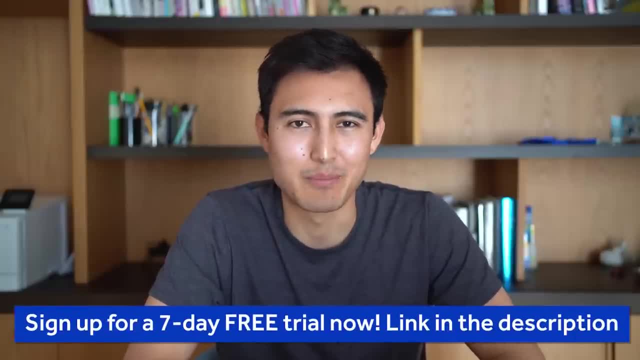 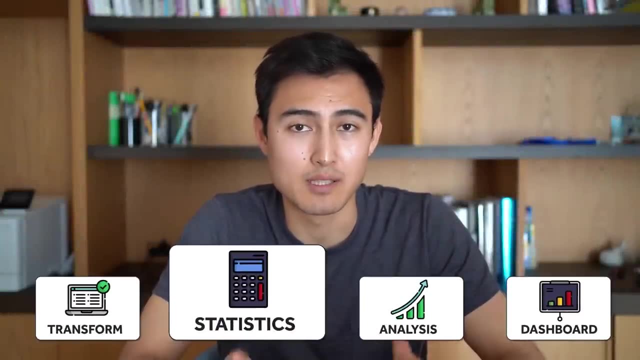 seven day free trial now using the link in the description below. all right back to the video. great, now that we've done step one and step two, it's all about the descriptive statistics, so really seeing things like: what's the average price? what about the minimum, the maximum? 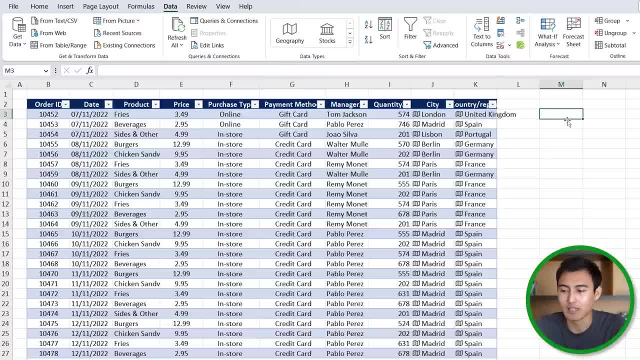 and so on. so for this let's hop over to the side and you could try to find for the price and for the quantity, say the average, going one by one. so type the average formula, then doing the same thing with the minimum, the maximum, so on. but there is a much faster way. that's actually using a tool called data. 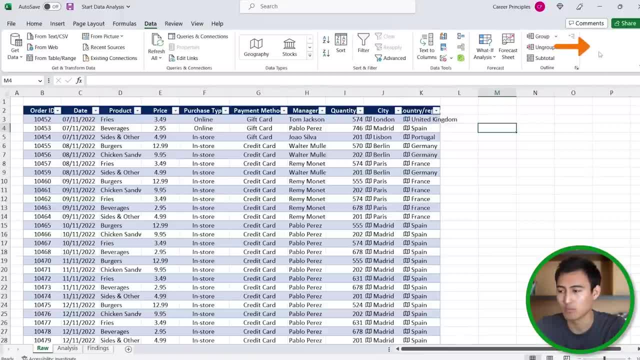 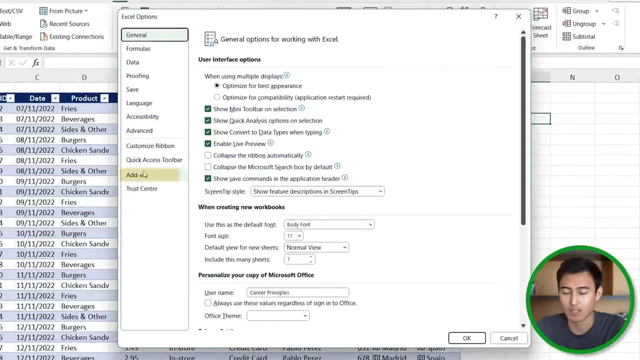 analysis. for that we're gonna have to activate it. it should be over here to the side under the data ribbon. if you don't have it, like me, we can go ahead and activate it. so we'll head over to file. go over to the bottom where it says options. from here we're gonna go into add-ins. 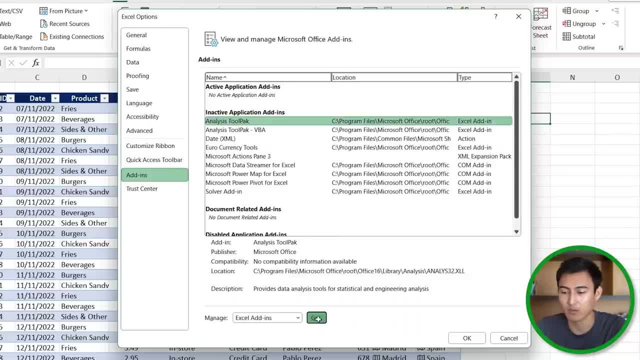 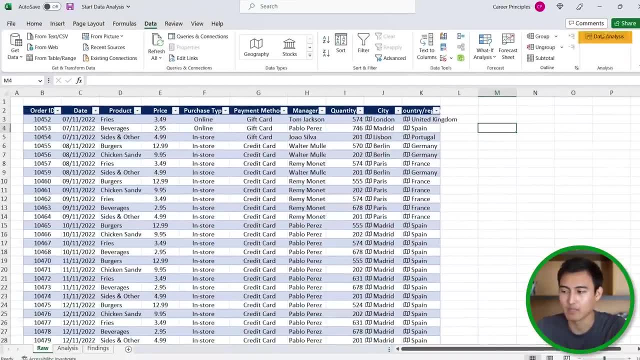 and we wanna click on the analysis tool pack here and hit on go from here. we wanna select analysis tool pack, like i said, and we'll hit ok. now you can see that we have this data analysis option under the data ribbon, so that's the one that we want to select. 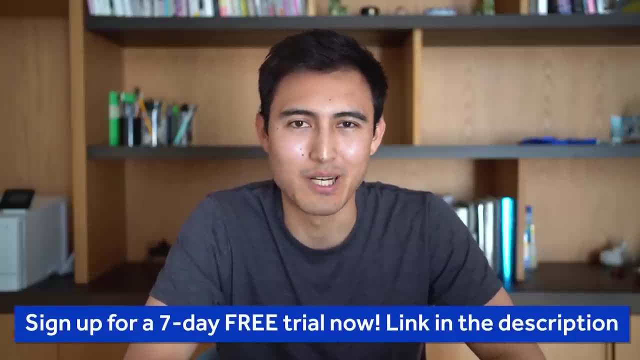 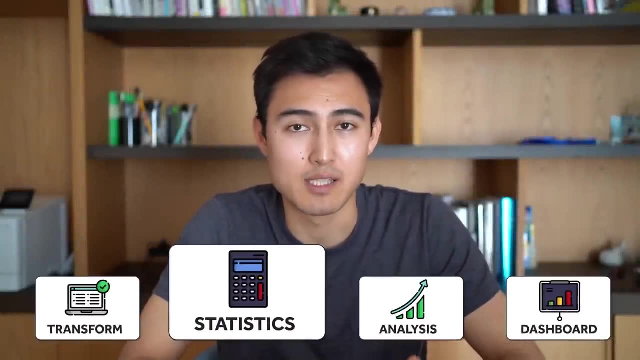 seven-day free trial now using the link in the description below. all right back to the video. great, now that we've done step one and step two. it's all about the descriptive statistics, so really seeing things like: what's the average price? what about the minimum, the maximum? 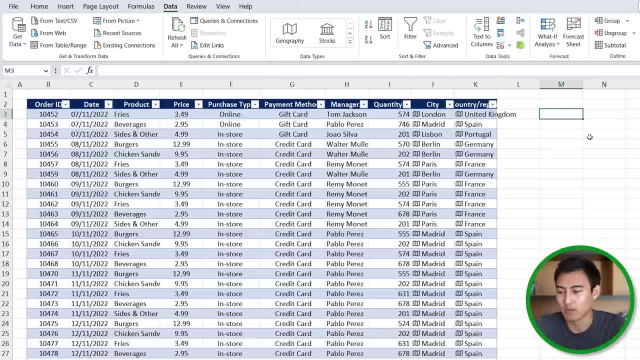 and so on. so for this let's hop over to the side and you could try to find for the price and for the quantity, say the average, going one by one. so type the average formula, then doing the same thing with the minimum, the maximum, so on. but there is a much faster way. that's actually using a tool called data. 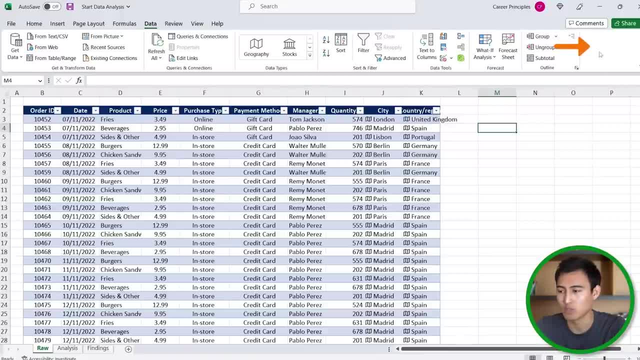 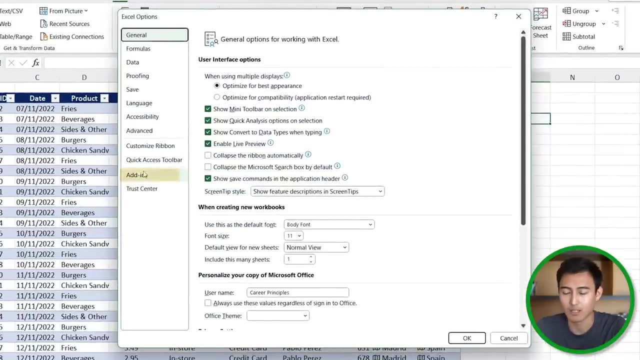 analysis. for that we're gonna have to activate it. it should be over here to the side under the data ribbon. if you don't have it, like me, we can go ahead and activate it. so we'll head over to file. go over to the bottom where it says options. from here we're going to go into add-ins. 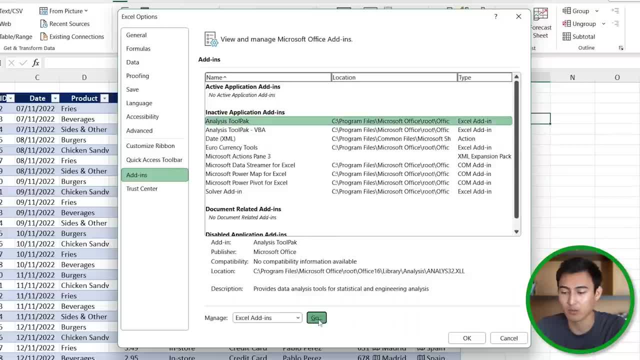 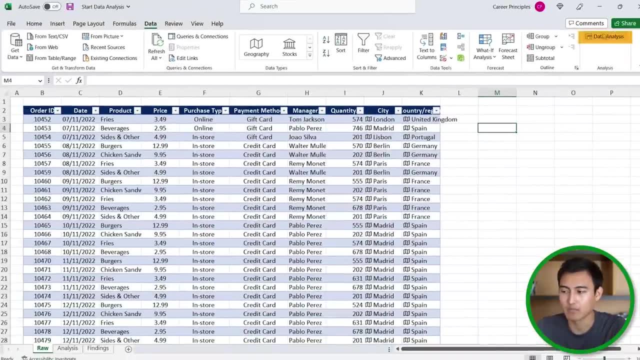 and we want to click on the analysis tool pack here and hit on go from here. we want to select analysis tool pack, like i said, and we'll hit ok. now you can see that we have this data analysis option under the data ribbon, so that's the one that we want to select. 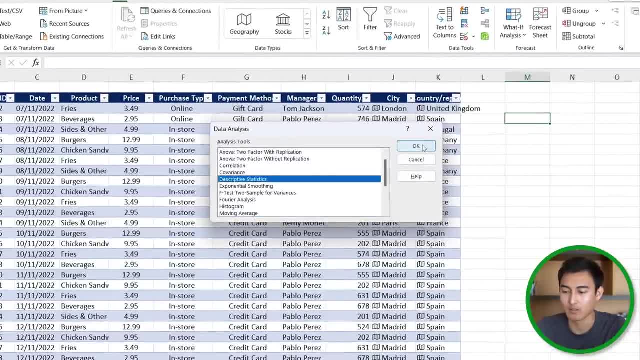 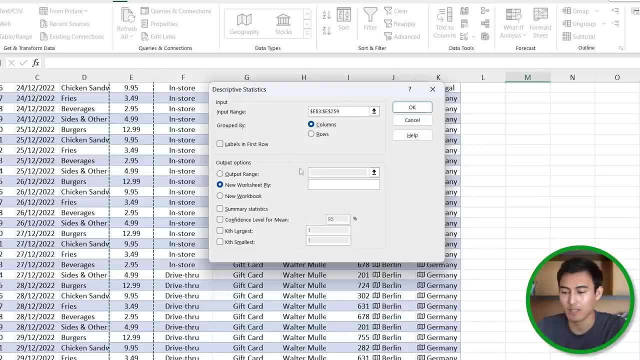 from here. we want the descriptive statistics and we'll hit on ok there and the input range is going to be all of our prices, so we'll go ctrl shift down there and then we want it to be a summary statistics. and where do we want this? let's say we want an 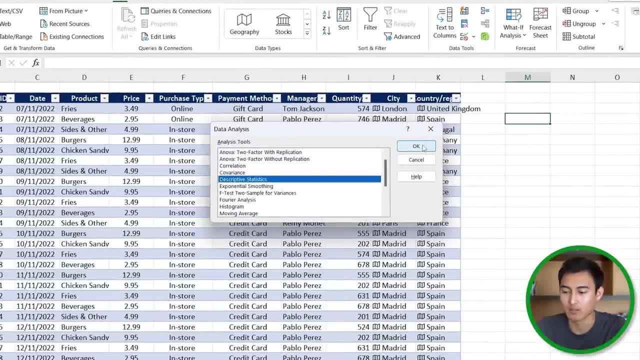 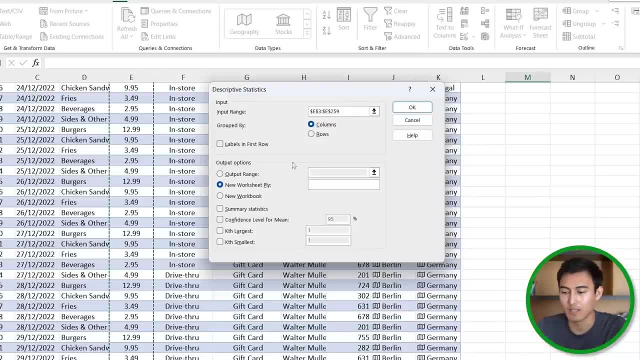 from here. we want the descriptive statistics and we'll hit on ok there and the input range is going to be all of our prices, so we'll go ctrl shift down there and then we want it to be a summary statistics. and where do we want this? let's say we want an 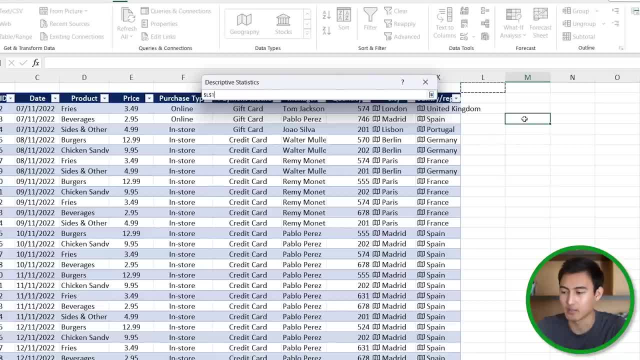 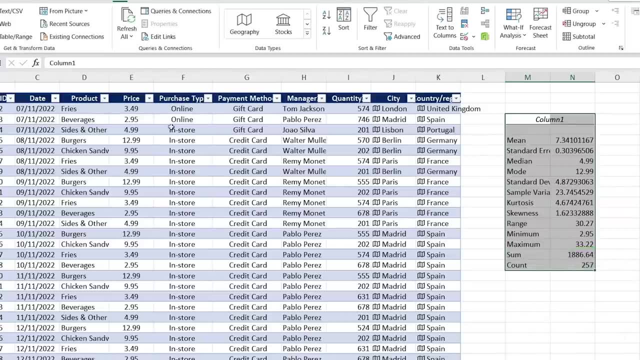 output range which is going to be up over here, so right next to the table. let's say, we put it here, to the side, there we're just going to hit on. ok, and now you can see that for the price, which is what we've selected, we've gotten everything from the mean, the median mode. 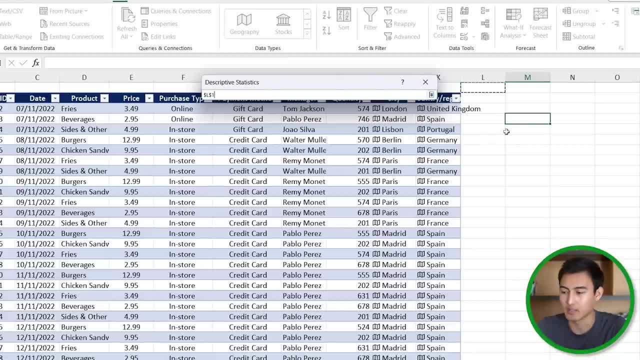 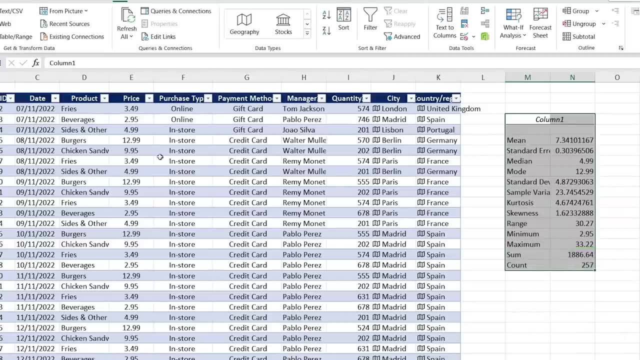 output range which is going to be up over here, so right next to the table. let's say, we put it here, to the side, there we're just going to hit on. ok, and now you can see that for the price, which is what we've selected, we've gotten everything from the mean: the median mode, minimum, maximum sum. 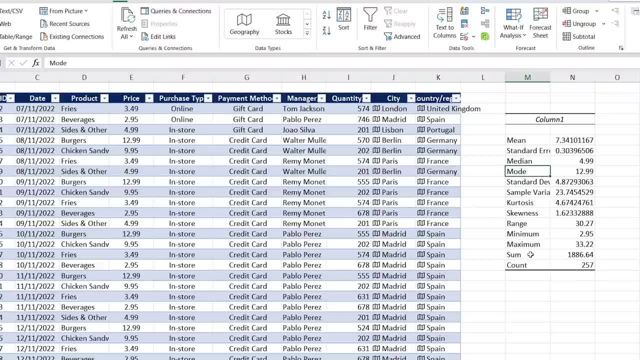 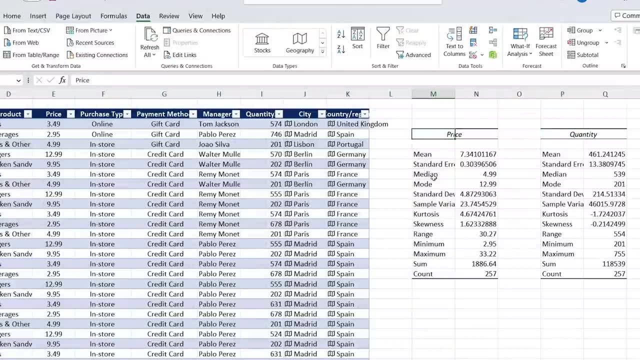 of other useful information. let me repeat that same process for the quantity. awesome, now we've got the breakdown by price and by quantity as well, but one thing that this doesn't quite account for is the fact that there could be outliers in our price, so for that we can go ahead down over here. 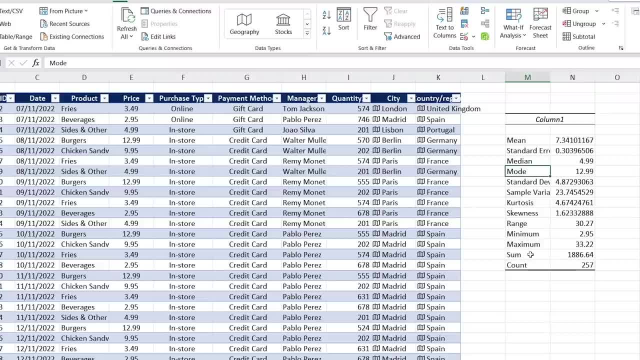 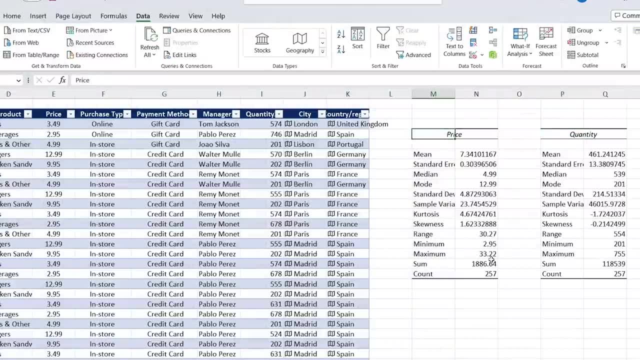 minimum maximum sum and a bunch of otherì useful information. Let me repeat that same process for the quantity. Awesome, now we've got the breakdown by price and by quantity as well, but one thing that this doesn't quite account for is the fact that there could be outliers in our price, So for that we can go ahead down over here. 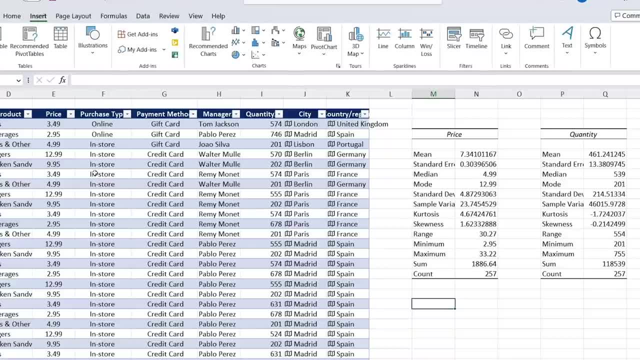 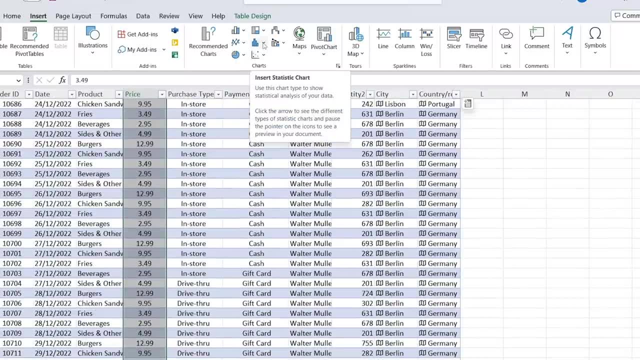 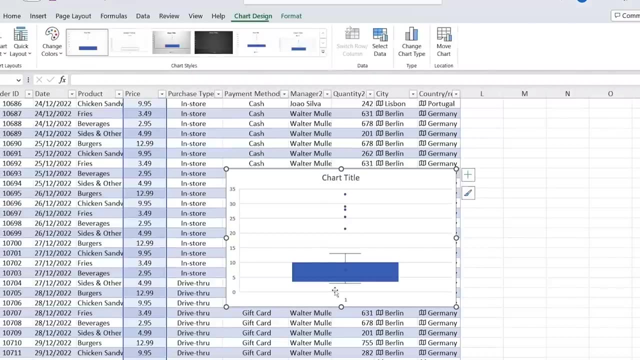 we're going to basically create a new chart which is going to be a box and whisker. So let's first select all of the prices. so ctrl shift down and down over here. you're going to find this icon. click on that and we want a box and whisker, basically this one over here and don't worry, 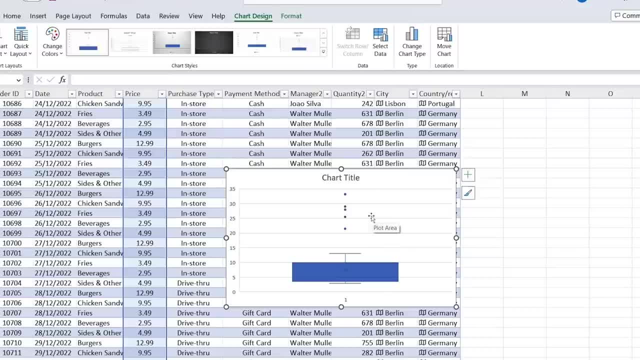 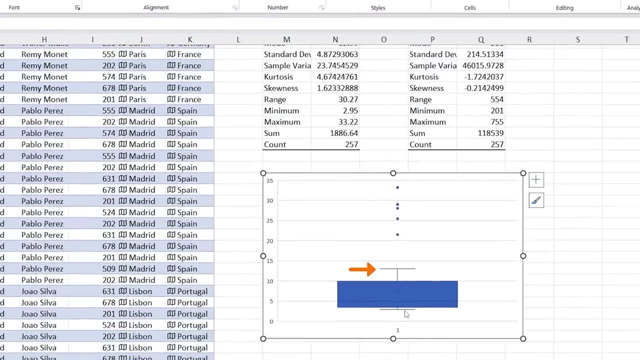 if you can't interpret it, we'll look at it just in a second. let me move that all the way up. So once we have it in here, this is basically telling us a few different things. so first, these top and bottom lines are telling us the maximums, so the max and the min, if you will, and then in 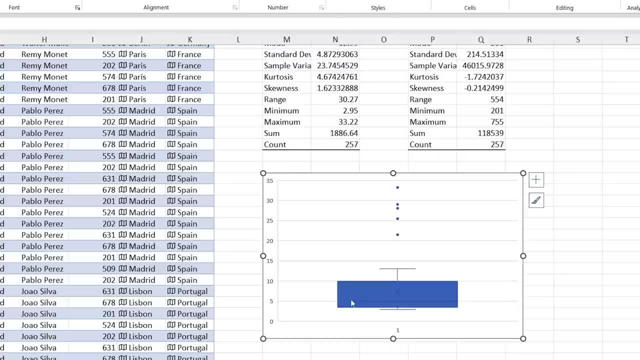 here. this box represents the first and the third quartile, and then you can see that we've got the x, which is the average, then we've got a line which is going to be the median, and finally we've got these dots over here which represent all of our 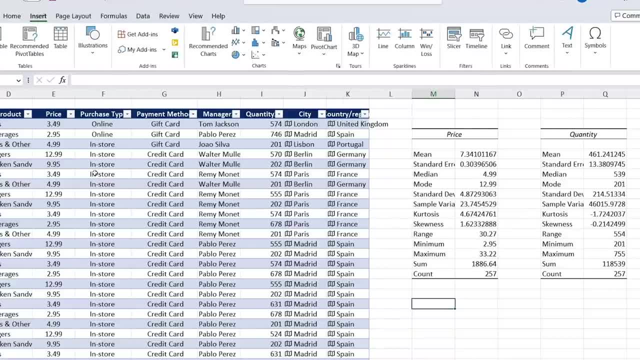 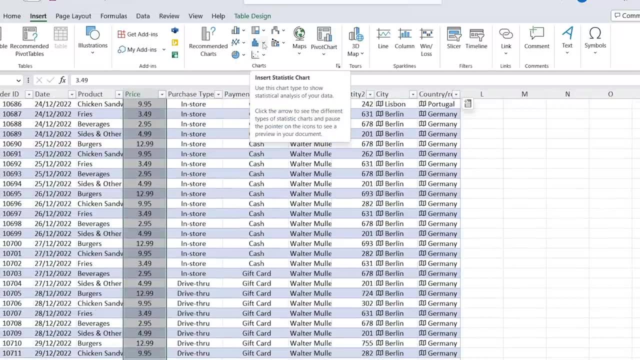 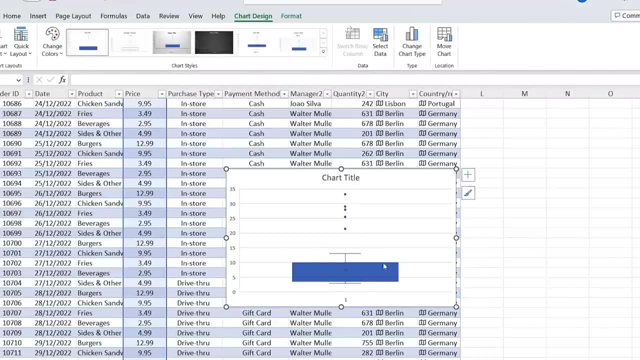 we're going to basically create a new chart which is going to be a box and whisker. so let's first select all of the prices. so control, shift down and down. over here you're going to find this icon. click on that and we want a box and whisker, basically this one over here and don't worry, 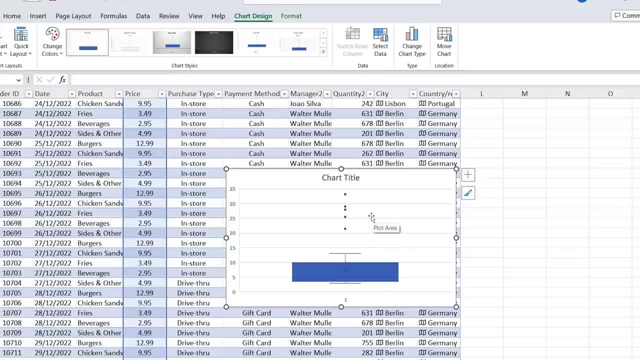 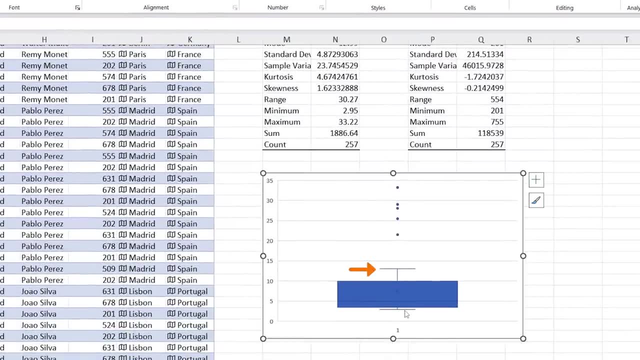 if you can't interpret it, we'll look at it just in a second. let me move that all the way up. so once we have it in here, this is basically telling us a few different things. so first, these top and bottom lines are telling us the maximums. so the max and the min. 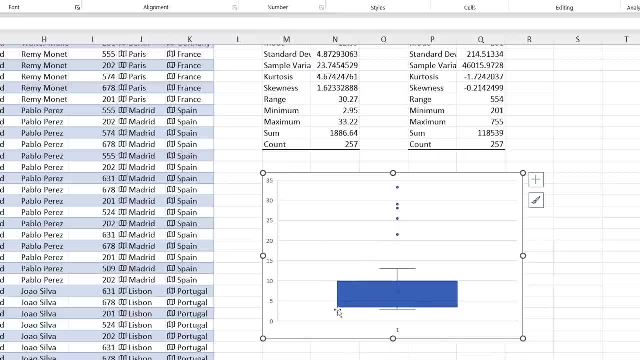 if you will, and then in here this box represents the first and the third quartile, and then you can see that we've got that x which is the average, then we've got a line which is going to be the be the median and finally we've got these dots over here which represent all of our outliers. 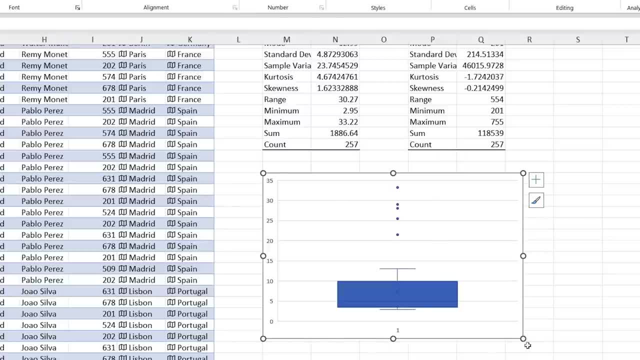 in our price. now, if we want to dig a bit further into this, it would be nice to see the x-axis. maybe we can put something like the manager's name to see where exactly this is coming from. maybe it's one manager that might be reporting the data wrong, so we'll go to right click for. 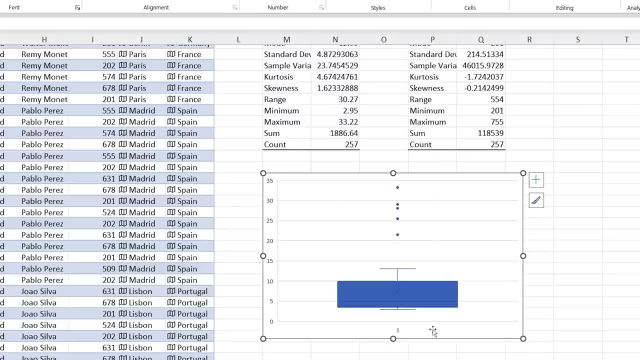 outliers in our price. Now, if we want to dig a bit further into this, it would be nice to see the x axis. maybe we can put something like the manager's name to see where exactly this is coming from. maybe it's one manager that might be reporting the data wrong, So we'll go to right click for. 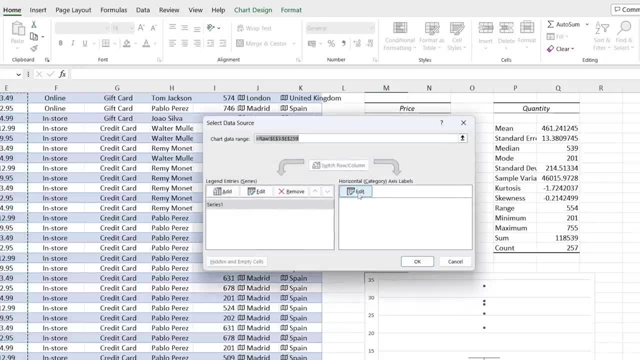 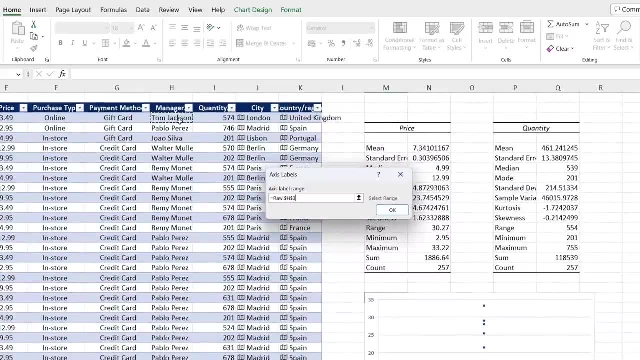 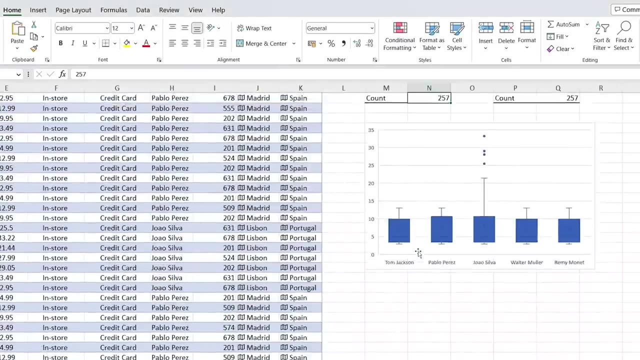 that go under select data, edit the horizontal category access label here, and what we're gonna put the managers. so we're gonna select all of these ctrl, shift down and hit on okay, and hit on okay again. Now, if we go all the way back up, you can see what that breakdown looks like by manager. 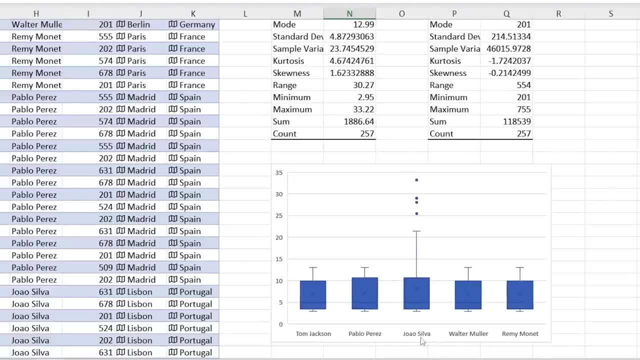 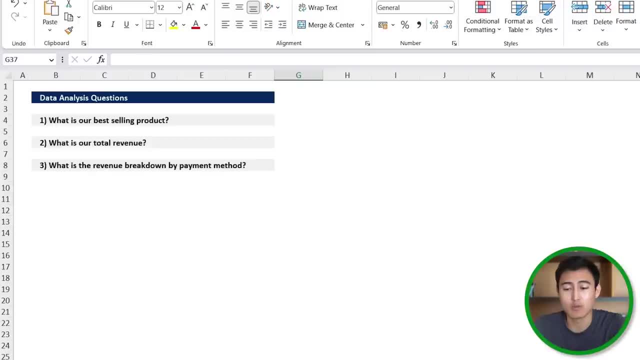 and it seems to be that all of these outliers are accumulated with Joao. maybe we should have a word with him Now, moving on to step three, which is data analysis. So over here you can see that we've got three different questions that we want to solve, which is, what is our best selling product? 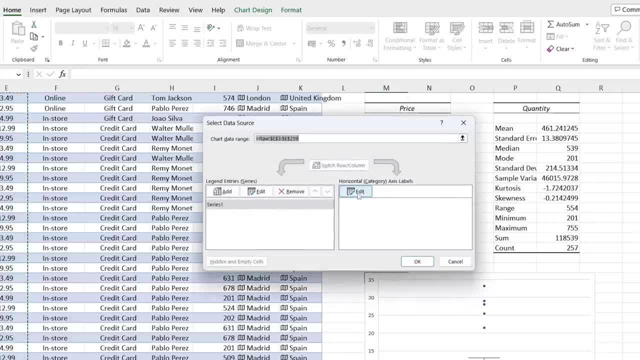 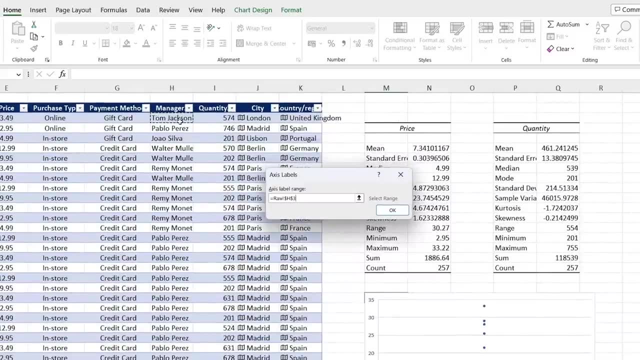 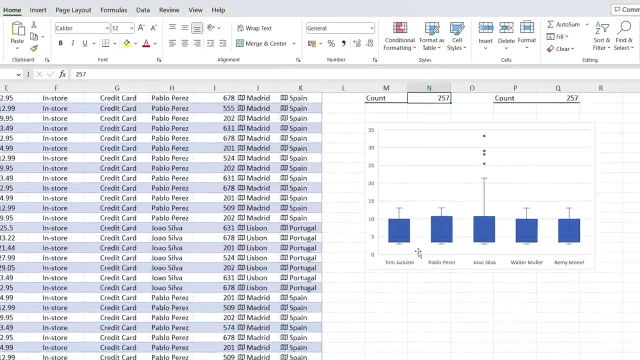 that go under select data, edit the horizontal category access label here, and what we're gonna do? the managers. so we're gonna select all of these control, shift down and hit on ok, and hit on ok again. now, if we go all the way back up, you can see what that breakdown looks like by manager. 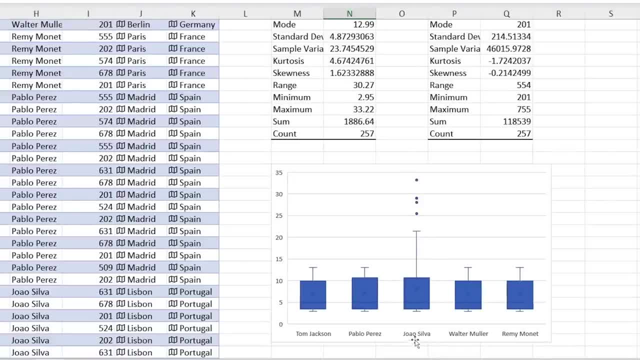 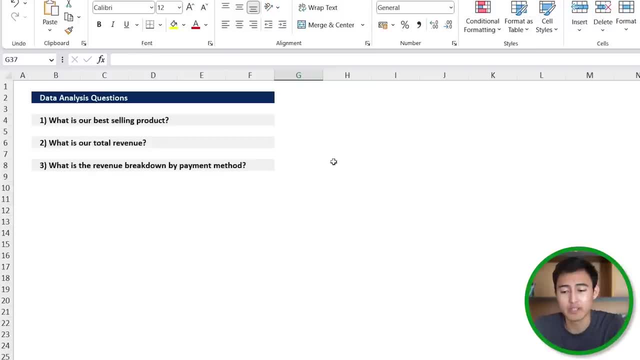 and it seems to be that all of these outliers are accumulated with joao. maybe we should have a word with him now, moving on to step three, which is data analysis. so over here you can see that we've got three different questions that we want to solve, which is, what is our best selling product? 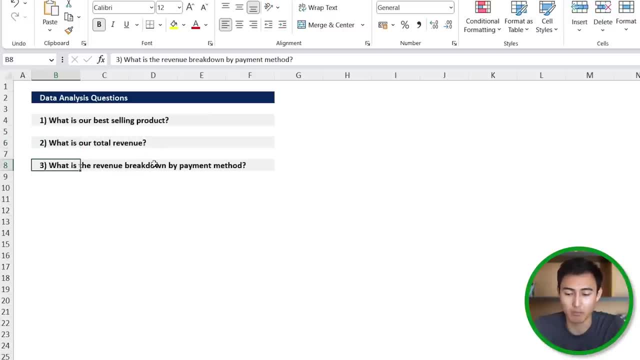 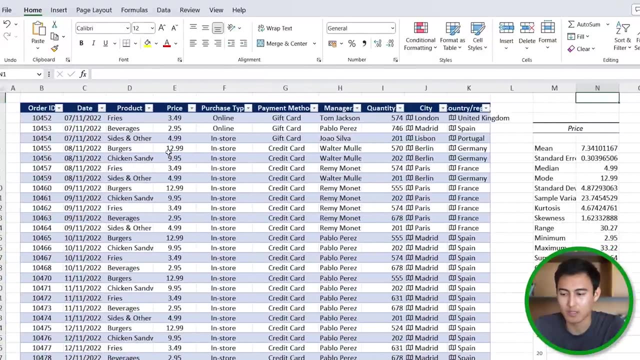 what is our total revenue and that's what's our revenue breakdown by payment method. so if we go back to the table here, you'll notice that we don't actually have a column for revenue, so that's one that we're gonna have to calculate simply by multiplying the price and the quantity. so we'll 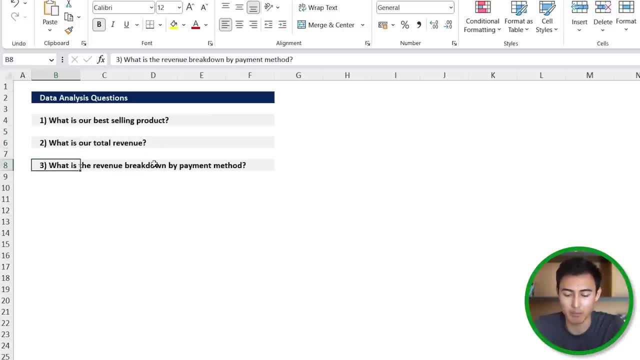 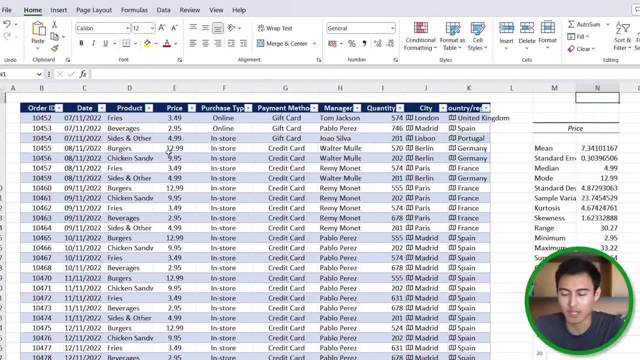 what is our total revenue and that's what's our revenue breakdown by payment method. So if we go back to the table here, you'll notice that we don't actually have a column for revenue, so that's one that we're gonna have to calculate simply by multiplying the price and the quantity. So we'll 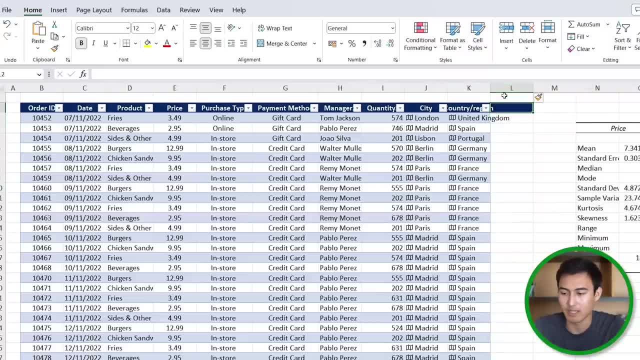 do that over here. let me add an extra column there and let's call this something like a revenue, and the formula for it is gonna be: equals the quantity multiplied by the price, and we'll just give it an extra column here. that should be calculated for us, and then we'll go up over. 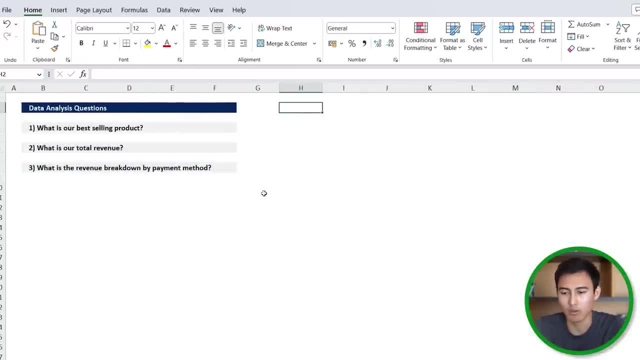 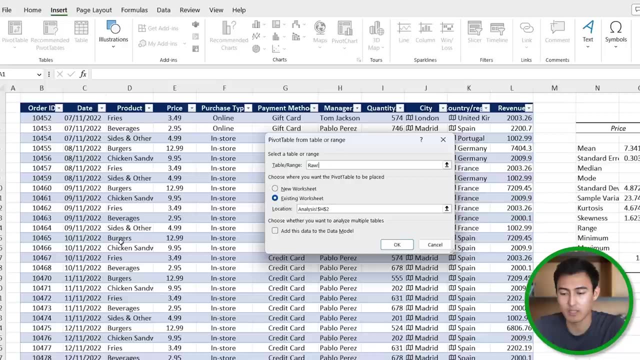 here again and for all of this analysis we can actually do most of it with a pivot table. So we'll head over to insert pivot table. The table or range we're interested in is all of this range. so once we select one of the cells, we can just go to ctrl a. that's going to select all of them. 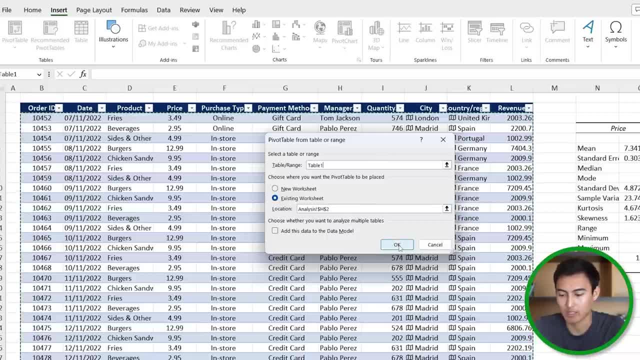 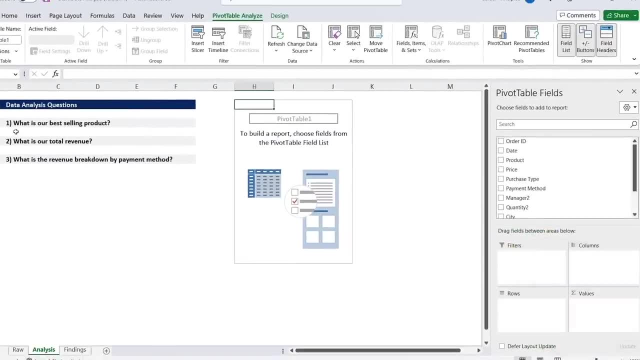 and we want this in a location in an existing worksheet which we already selected. so we'll hit okay. From here we can start doing all the breakdown. so what's our best selling product? so let's do this by quantity. we're going to select the products as the rows just hover that over and then we're. 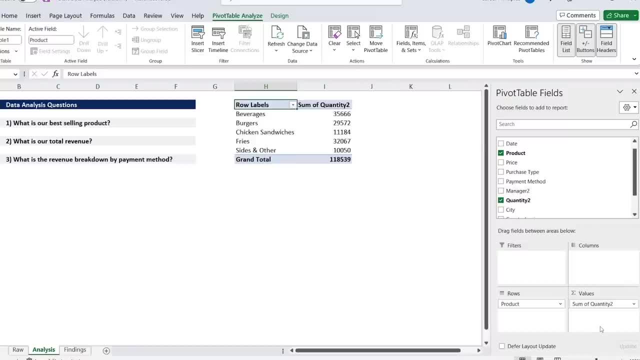 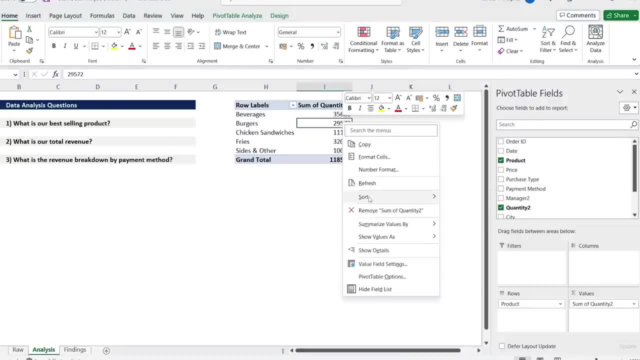 going to select the quantity over here as the values. Great, now we have all of that breakdown. if we want to sort it from highest to lowest, we can go to right click and go to sort and we'll sort largest to smallest. and now you can see that beverages is our largest at 35 000. 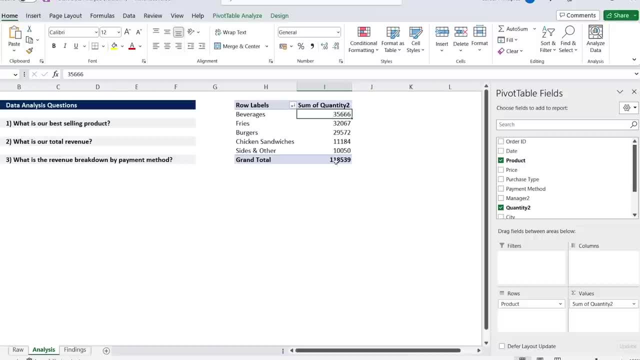 Then, secondly, we've got what is our total revenue for this one. we're simply gonna have to select the revenue. so first we'll remove these, let's take this out, and we'll take this out as well- and we just have to select the revenue and put it under values that should give us the sum of total. 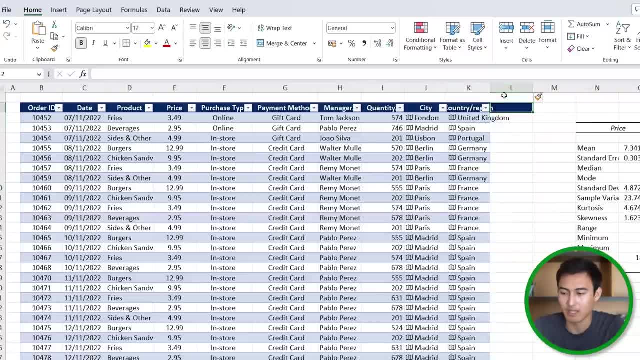 do that over here. let me add an extra column there and let's call this something like a revenue, and the formula for it is gonna be: equals the quantity multiplied by the price, and we'll just hit enter there. that should be calculated for us, and then we'll go up over here again and for all of 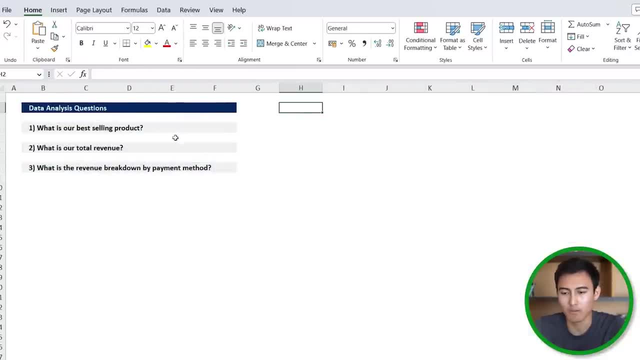 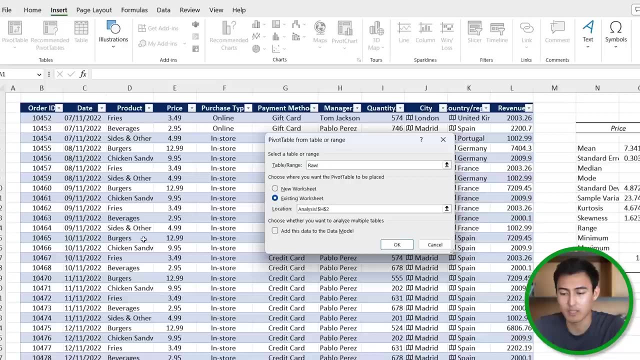 this analysis. we can actually do most of it with a pivot table, so we'll head over to insert pivot table. the table or range we're interested in is all of this range. so once we select one of the cells, we can just go to control a that's going to select all of them, and we want this in a location. 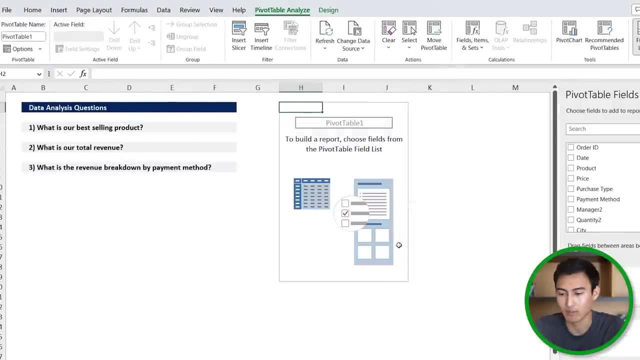 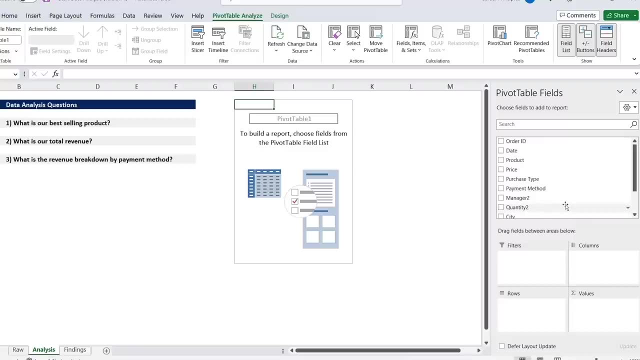 in an existing worksheet which we already selected. so we'll hit: ok, great, here we can start doing all the breakdown. so what's our best selling product? so let's do this by quantity. we're going to select the products as the rows just hover that over, and then we're 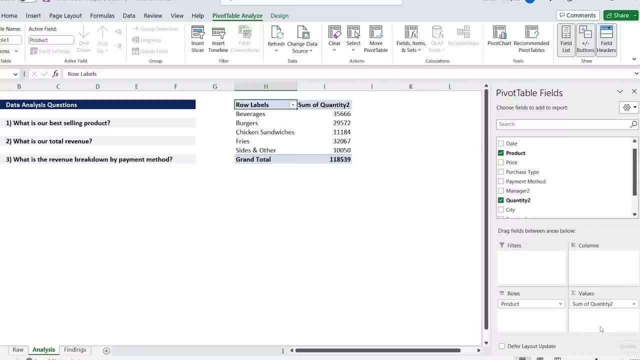 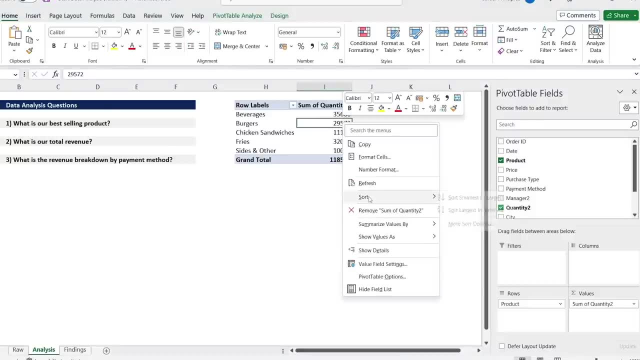 going to select the quantity over here as the values. great. now we have all of that breakdown. if we want to sort it from highest to lowest, we can go to right click and go to sort and we'll sort largest to smallest. and now you can see that beverages is our largest at 35 000. 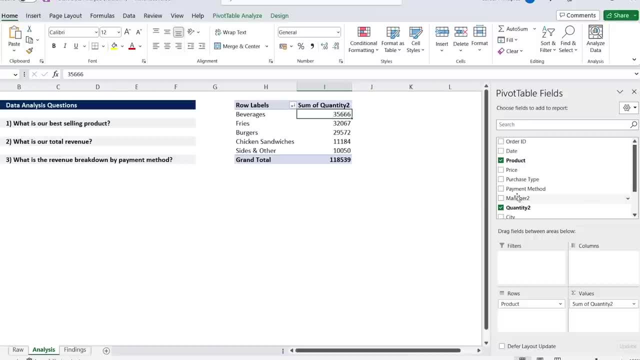 secondly, we've got what is our total revenue for this one. we're simply gonna have to select the revenue. so first we'll remove these, let's take this out, and we'll take this out as well- and we just have to select the revenue and put it under values that should give us the sum of 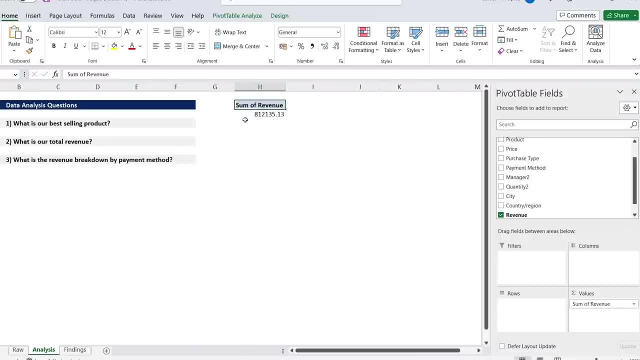 total revenue, which seems to be 812 000, and finally our revenue breakdown by payment method. so for that we're gonna get all of the payment methods and put those under the rose, like so, but to see the breakdown better, it probably makes more sense as a percentage. 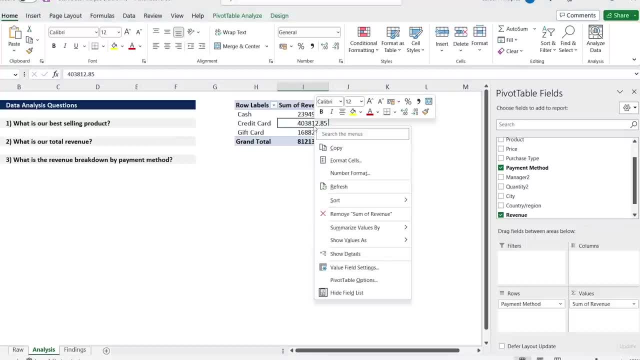 so what we can actually do is go to right click and from here go to summarize- show values- us sorry- and we're going to show them as a percentage of the grand total. now you can see that full breakdown and it seems like credit cards are the most dominant here. now that you've seen how 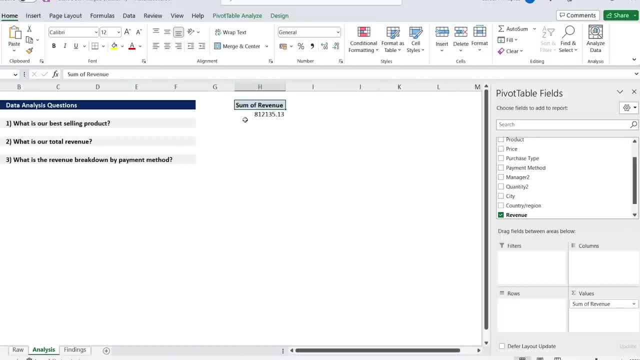 revenue, which seems to be eight hundred and twelve thousand, and finally our revenue breakdown by payment method. so for that we're gonna get all of the payment methods and put those under the rose like so, but to see the breakdown better, it probably makes more sense as a percentage.